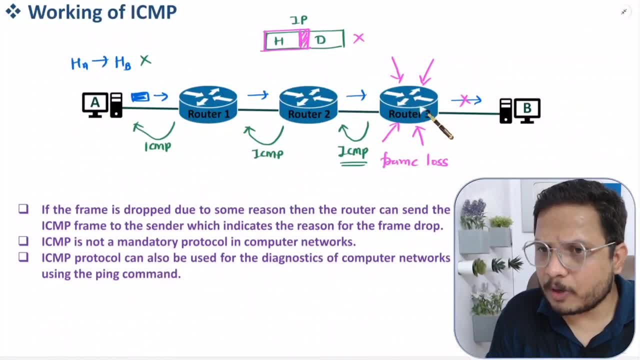 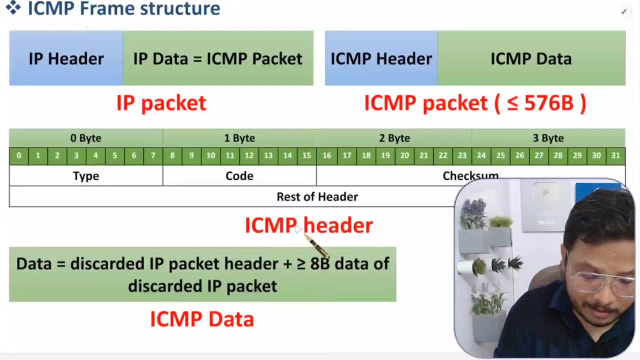 And I have told you like there can be so many reasons of frame drop. and in ICMP frame structure, I have told you in ICMP header this type and code field will define what is the reason behind frame drop. So you should know, see, in internet packet ICMP is implemented. 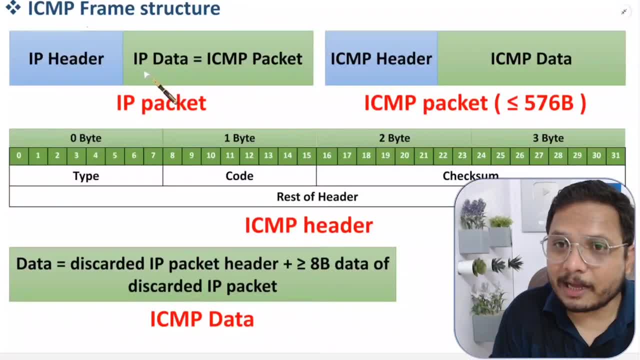 So in IP packet there can be IP header and IP data. Here, with IP data, we will be having ICMP packet. In ICMP packet we have ICMP header and ICMP data. ICMP header is having type and code field that will define what is the reason behind. 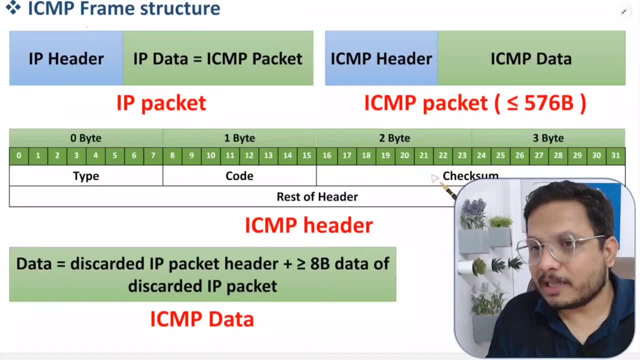 frame drop and checksum explains you whether there is error or not. And this rest of header that is not used. it will be usually zero in majority of cases And here ICMP data that will be discarded. packets header plus greater than 80% error. 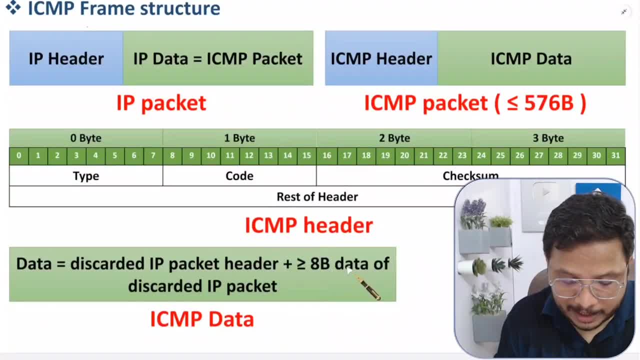 So this is the reason behind frame drop And check some explains you whether there is error or not. And this rest of header that is not used. it will be usually zero in majority of cases. So here ICMP packet is having 8 bytes of data from discarded packet. 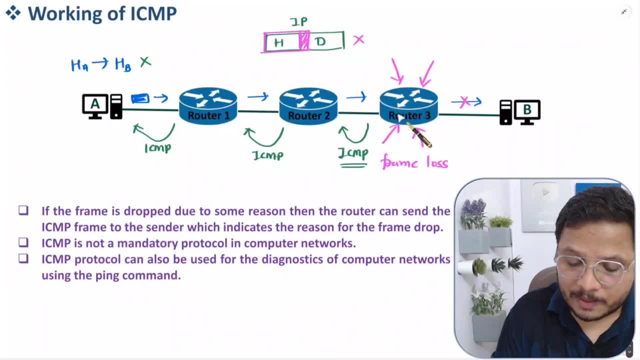 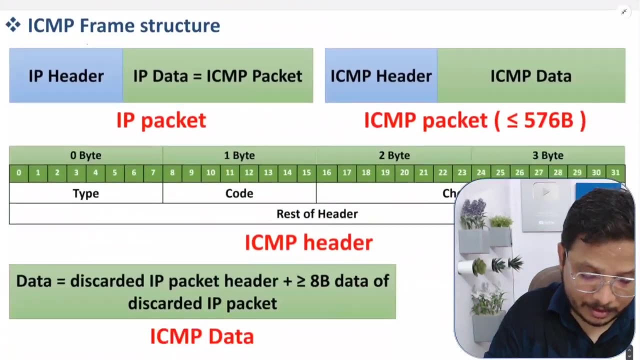 Like, for example, as if you transmit one frame and as if this frame is getting dropped over here, then with this frame, with this frame, we will be having header plus data. So here in ICMP, data header plus greater than 8 bytes of data that we are adding in. 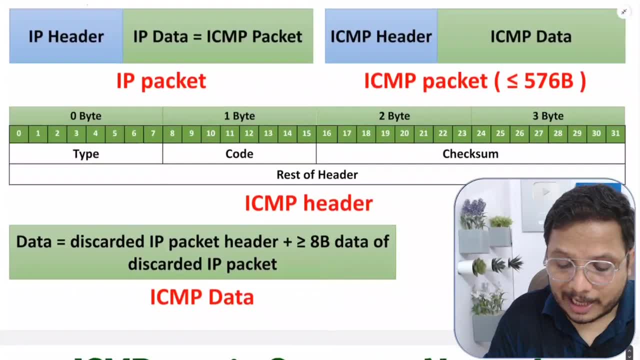 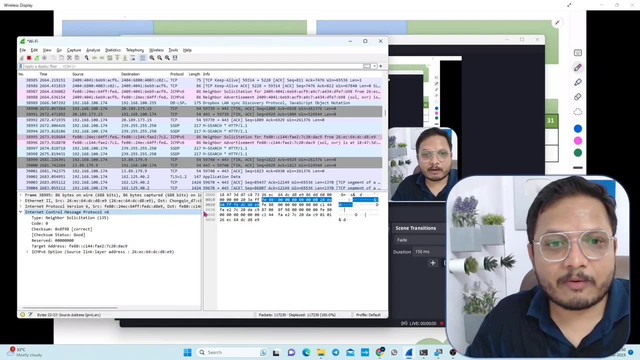 data part of ICMP data right. So in total ICMP packet is ICMP header plus ICMP data And that we include On ICMP packet. let me show you that practically So. for that I need to take to you my computer screen And in that if you observe here YR shark software that we have right. 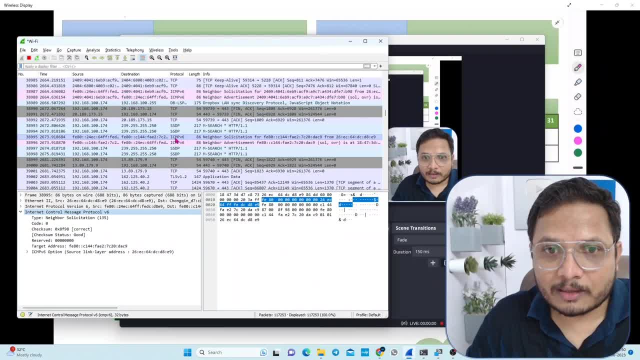 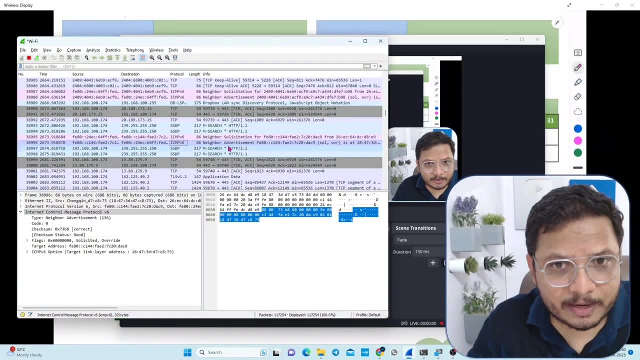 So here you see ICMP version six, this frame that I have received right And that is having neighbor solicitation, and second ICMP frame that I have received, that is neighbor advertisement. right Now, if you observe, if you click on this first, 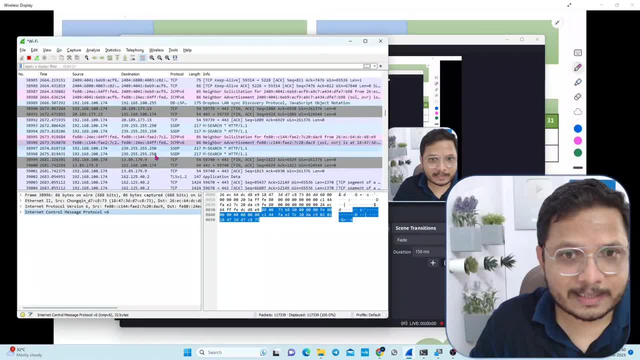 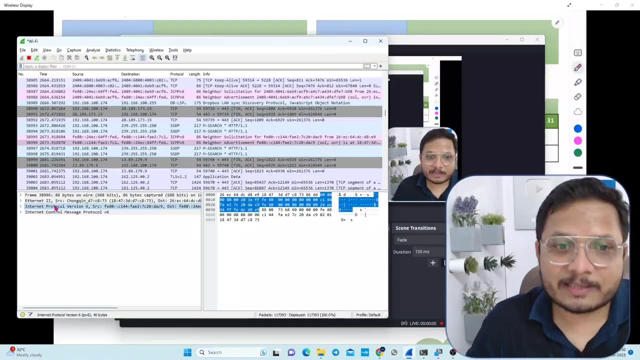 Then you will. details will be there with this frame, right, You see ICMP. ICMP means internet control message protocol. It is implemented on v6 right now with this frame. So here see this ICMP that is added on IPv6 frame. 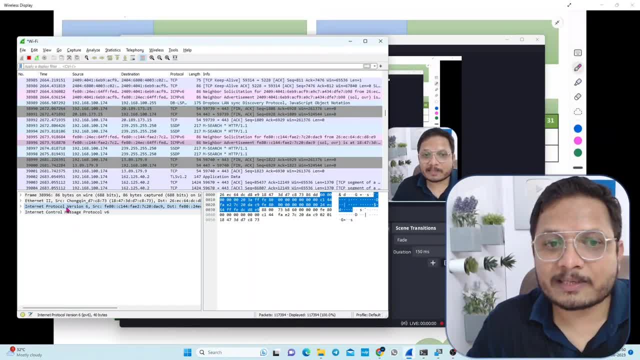 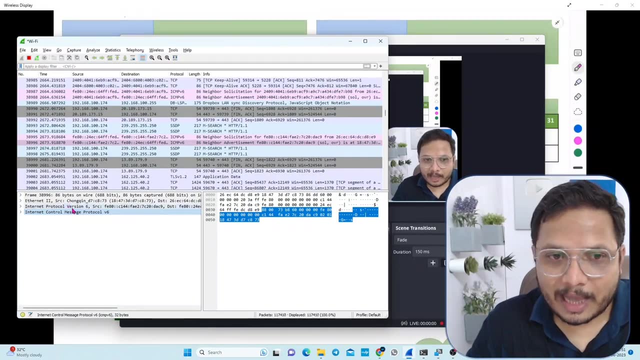 This is added on IPv6 frame. IPv6 is implemented on ethernet over here and ethernet is implemented as per frame structure over here, Right? So if you observe here ICMP, that is implemented along with IP protocol right on network layer. See, this is how things are there. 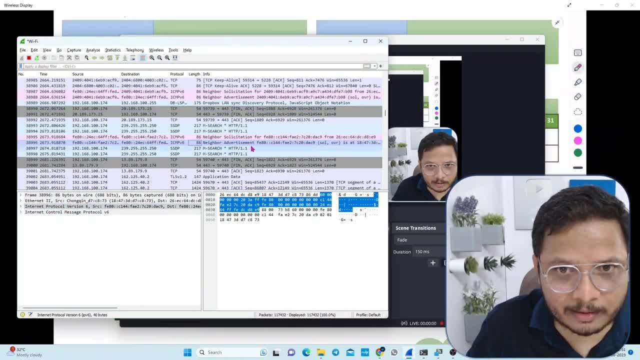 And here, if you observe what is this frame, you see neighbor advertisement right. So if you observe here, here we are having type and here we are having code, right, Checksum is there. checksum is there for error detection. 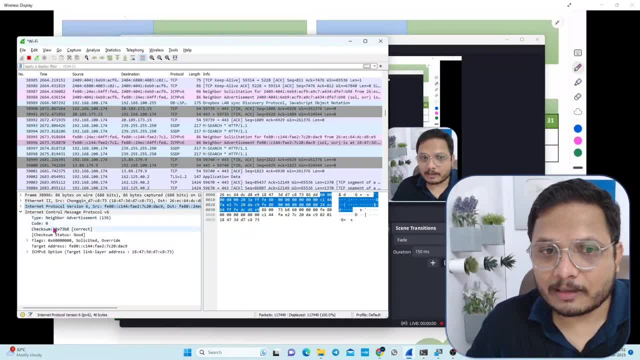 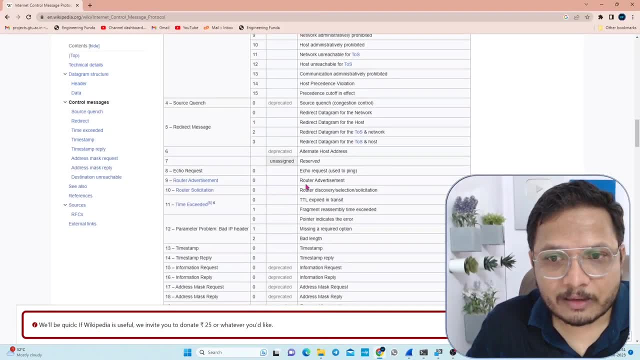 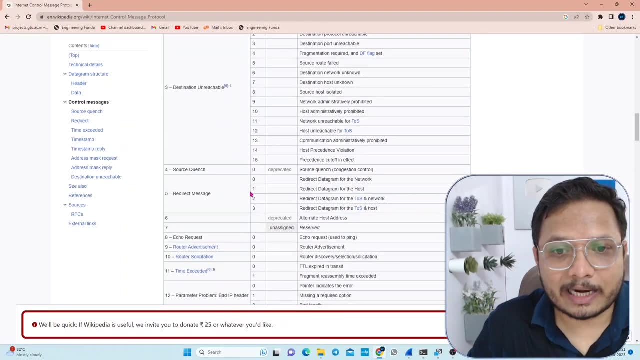 But type and code. that will explain the reason. So if you go through Wikipedia, let me show you in Wikipedia. in Wikipedia, if you observe, you see router advertisement that is having this type and this code. right, You see type and code that is written over here. 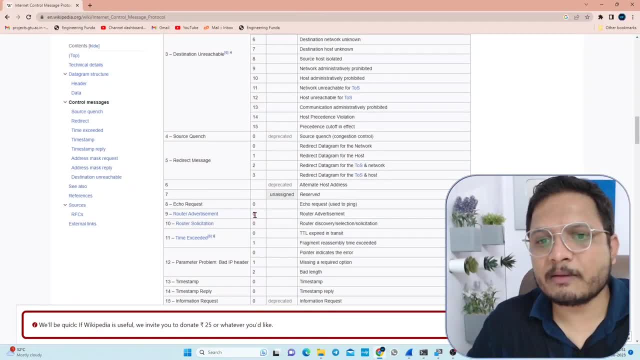 So this is, this is the detail which is there for IPv4.. But same thing that will be there for IPv6, only type and code that will change, Right, So here. So this is how things are there, right? So technically you can observe here how ICMP packet that is forwarded. 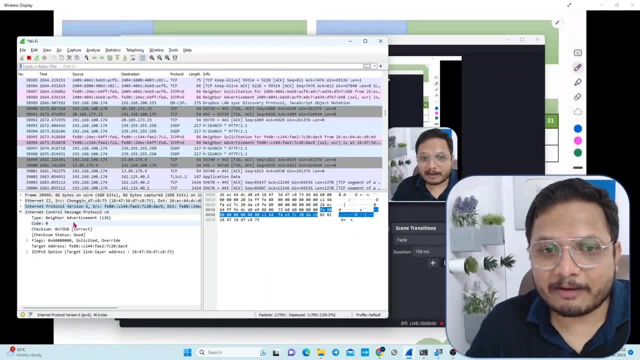 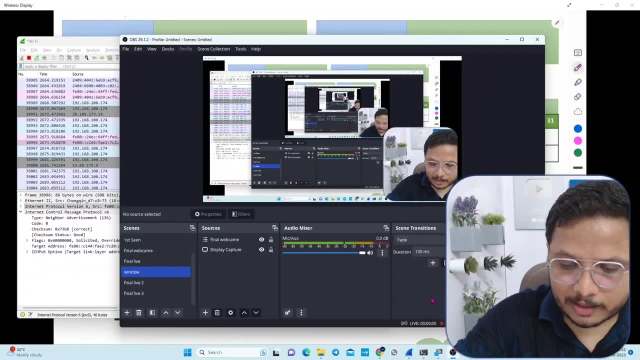 So type and code that explain the reason Here. neighbor advertisement. that is the reason. right Now. what I'll do is I'll explain you first. What I'll do is I'll explain you first how many, how many usages are there which I'm. 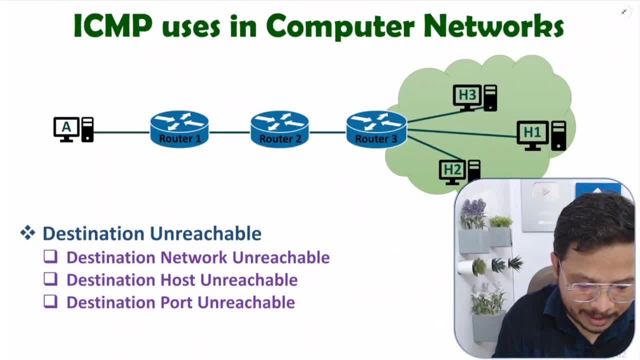 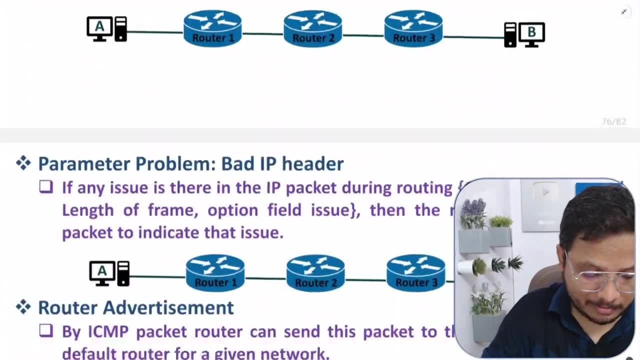 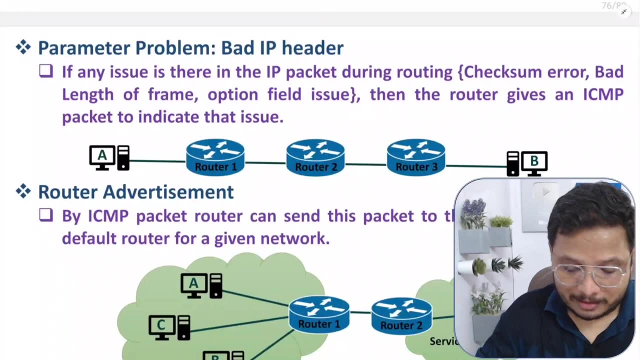 going to explain you in this video. see, there can be destination unreachable. there can be source quench. There can be time exceeded. There can be parameter problem like bad IP header. There can be router advertisement right. There can be router solicitation. 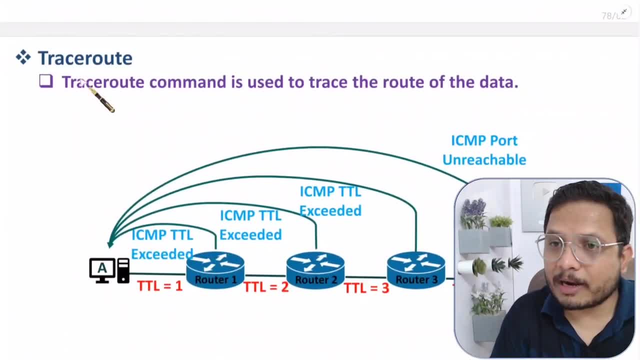 There can be ping command, There can be trace route command. So all this I'll explain you by practical examples right In my computer, along with wireshark software. So let us see first how destination unreachable that can be, there with us. 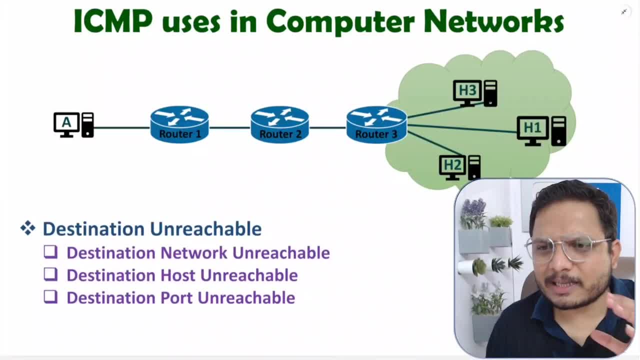 So here in destination unreachable. So here in destination unreachable In general. I'll explain you three categories right. One is destination network unreachable. Second is destination host unreachable. And third is destination port unreachable. Let me explain you that by practical example. 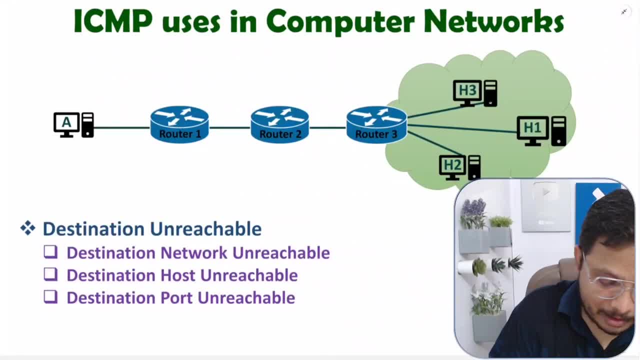 Like as if I say: here we are taking one example in which see: host A is forwarding data to host H1, right, So host A is forwarding data to host H1.. So host A is forwarding data to host H1.. So what will happen in case of network unreachable? 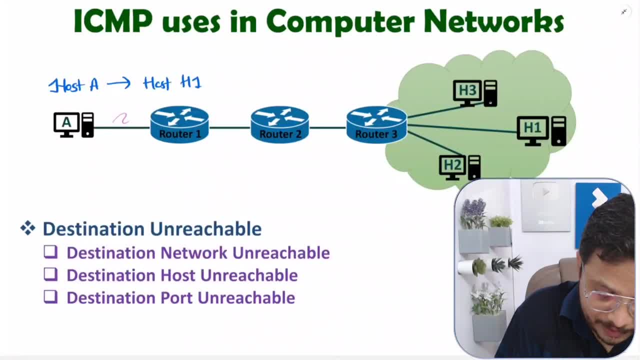 Let us try to understand that. You see here: first frame will go from A to router 1.. Then frame will go from router 1 to router 2.. Now you see, router 2 will forward data to router 3.. And router 3 belongs to network of host H1.. 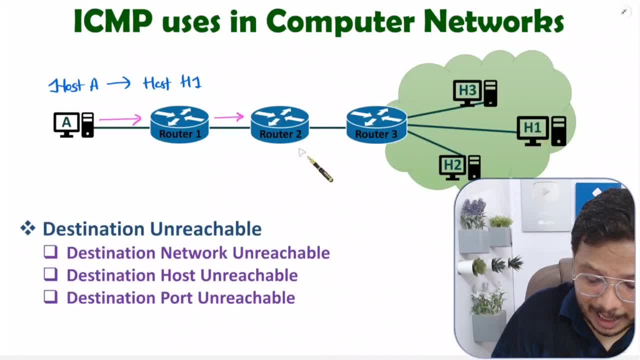 Router 3 belongs to network of host H1. And as if, As if router 2 does not find router 3, then you can say: here: destination network is unreachable. I'll show you that in Wikipedia even, But right now you just understand this. 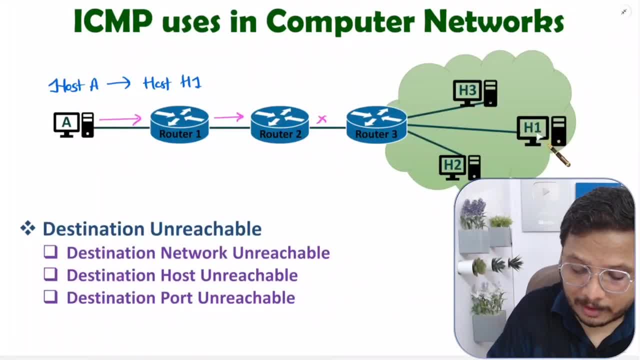 See, as if you want to communicate from host A to host H1 and as if this network is unreachable, then this router 2, you see, is finding this. router 3 is not reachable, So it will forward. So it will forward ICMP packet. 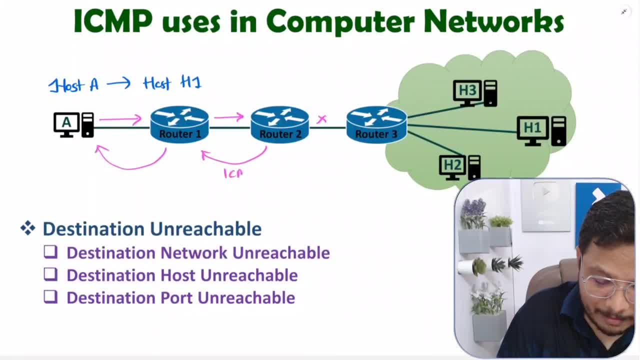 It will forward ICMP packet like this And in ICMP packet, in ICMP packet, it will mention this: This network is unreachable. right Now let me consider second case. In second case you see, destination host is unreachable. So destination host is unreachable means what? when you forward frame? when you forward frame, 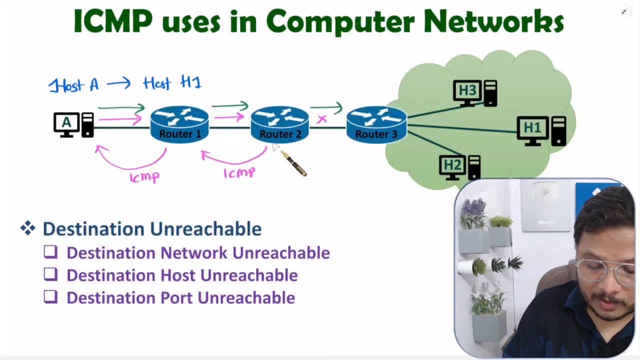 right At that time, Post Post and content is unreachable. So you see, frame will be routed to router one, then router one will route it to router 2.. Now router 2 will route it to router 3.. Now router 3, router 3 can communicate in this network. 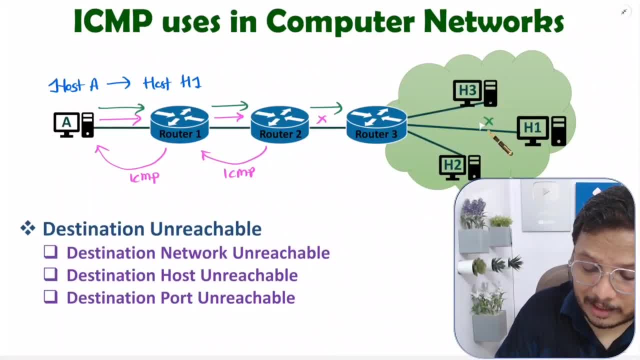 But in this network, as if this host H1 is unreachable with router 3, then router 3 will do what Router 3 will forward ICMP frame Router will. router 3 will forward ICMP frame And then host group, Host group. 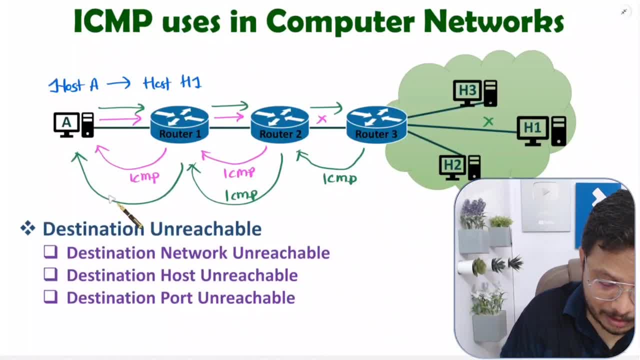 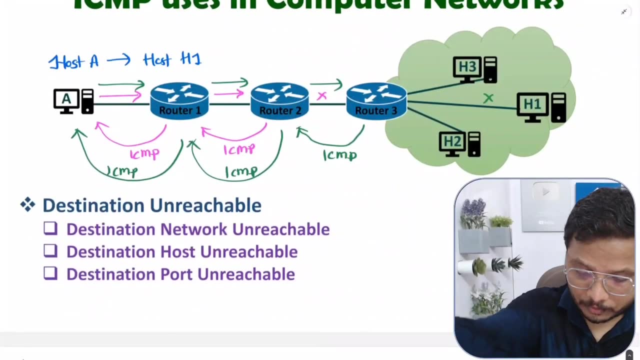 and it will mention, it will mention, it will mention what it will mention. this host is unreachable right now now, destination port unreachable. so that is quite interesting. you see what will happen here here, when host a is forwarding frame right to router 1, router 2, router 3, now it will reaches to h1. it will reaches to h1, but inside h1 there are multiple 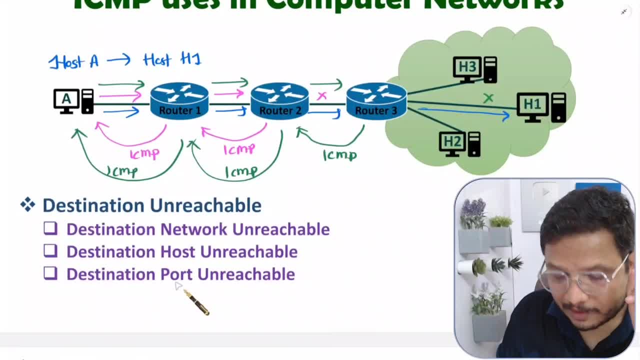 processes and with each process that will be, there will be well defined port number. like you may be using skype over here, right, let us say port 1, that is skype. let us say port 2, that is, that is google chrome. right, google chrome. likewise, there can be multiple ports now. for example, right now somebody is calling. 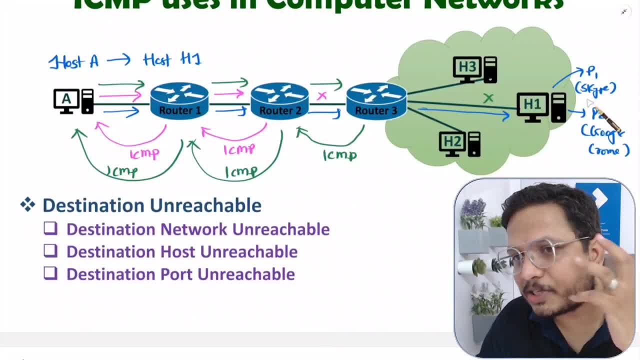 you on skype but your skype application is that skype application is not active on your host, then do you think like that somebody can talk to you by skype? no, so when frame comes over here addit, as if skype is not available over here on this host, then there will be. 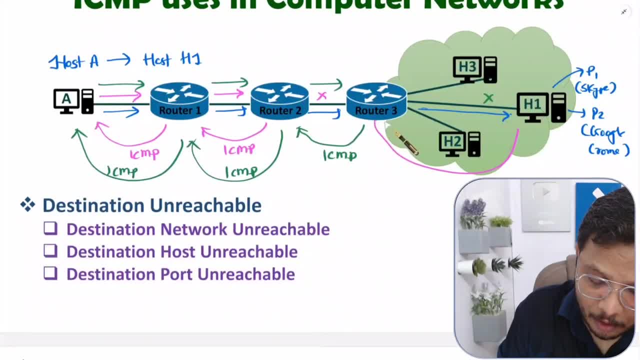 there will be. there will be ICMP. ICMP reply by host 1,. there will be ICMP reply by host 1,. right, that says port is port is unreachable. that says port is unreachable, right. see, that is how things will happen. 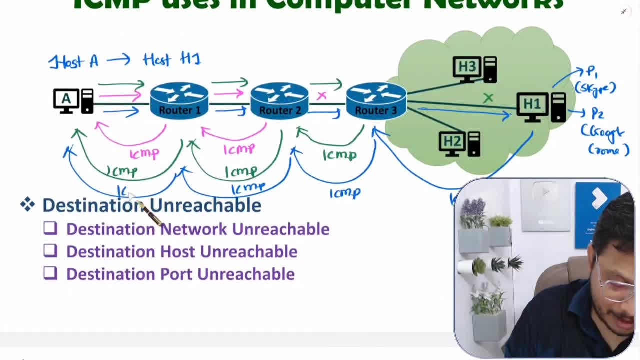 so I think now you are having fair enough idea like how, how network can be unreachable, how port can be unreachable, how host can be unreachable. now let me show you that on my computer screen so that will give you more clarity. like, if you observe here, Wikipedia: 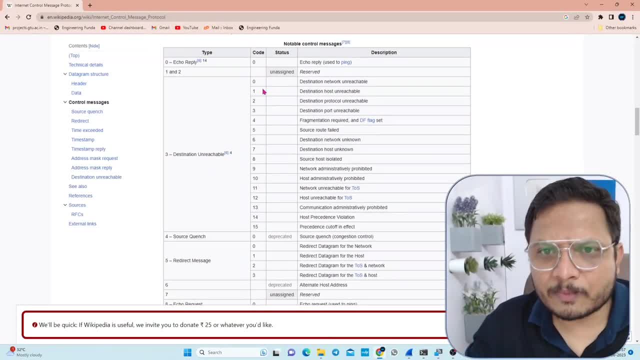 then, in that you see, destination unreachable is having so many types, right, destination unreachable is having so many types. like I have told you, network unreachable. like I have told you, destination host unreachable. destination protocol may be unreachable. destination port unreachable. sometimes there can be fragmentation required and DF flag is set to 1, see it. 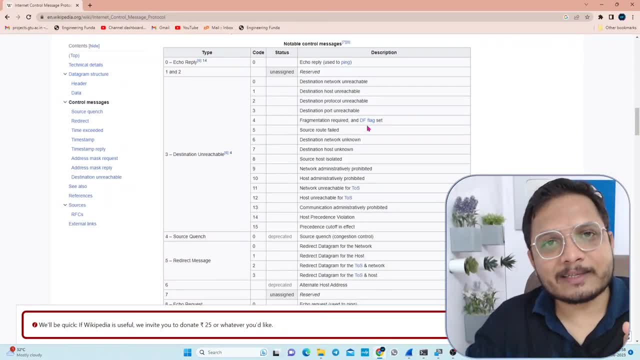 if DF flag, if it is set to 1, in that situation you cannot do fragmentation and as if fragmentation is not allowed, then ICMP reply will come like fragmentation required, but it is not allowed here. likewise, there are so many reasons right for destination unreachable, so I cannot. 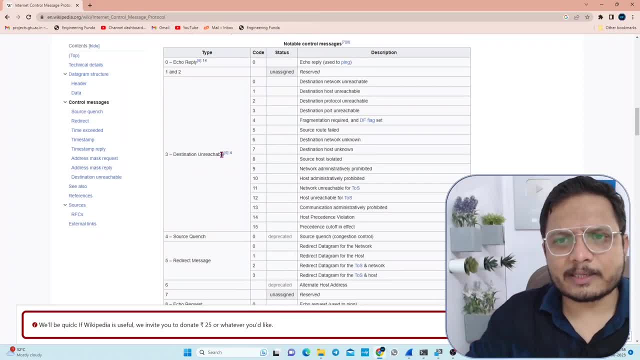 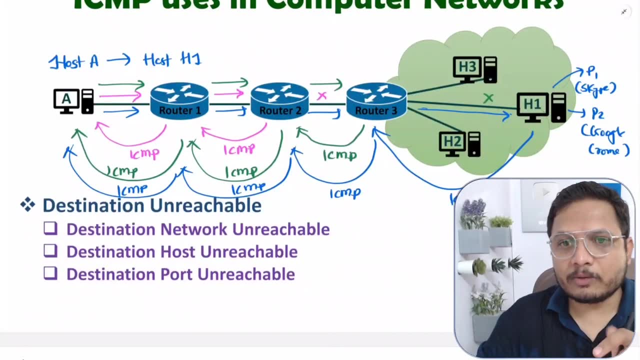 explain you all the reasons, but I have explained you general reasons. right, those are three general reasons. so here, I think now this part is clear. Let us move on to next part, that is source quench. so let us try to understand how source 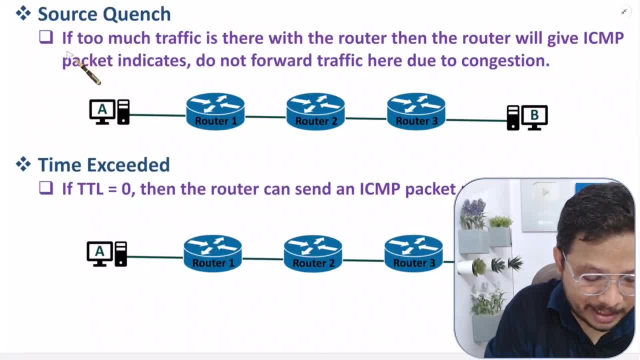 quench is there- see source quench. that is applicable. if too much traffic is there with router, then router will give ICMP packet indicates. do not forward traffic here due to congestion. let me explain you an example. like, for example, as if I say here router 3,. 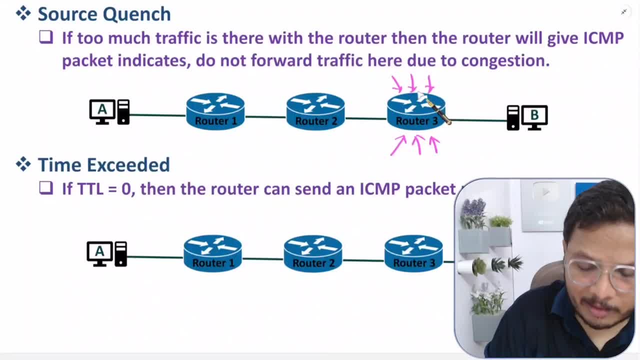 router 3, that is so busy. router 3 may be connected with so many LANs, Right, and that is why router 3 is very busy right now. and as if? as if host A is forwarding frame to host B and when frame comes to router 3, at that time router 3 may not be able to. 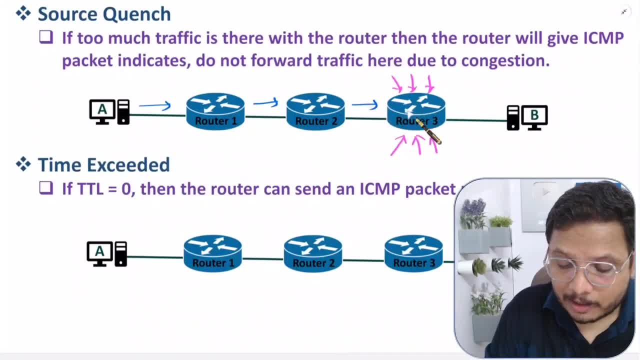 handle this frame. so router 3 will do what router 3 will give: ICMP packet over here. router 3 will give ICMP packet over here, right, and that ICMP packet, that ICMP packet, explains what That ICMP packet explains. right now this router 3 is very busy, so it will give so. 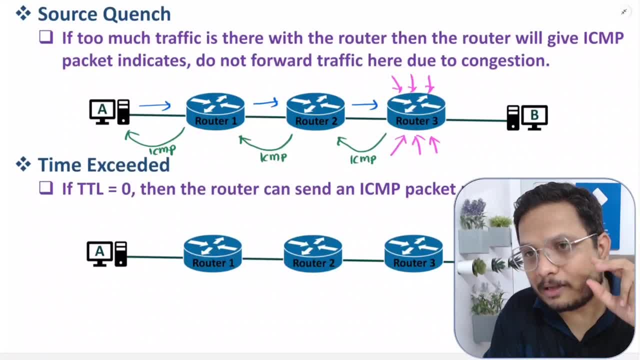 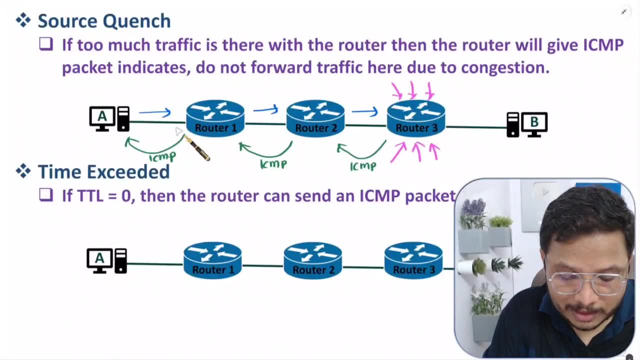 it will give command right in code and type field. it will give command which is source quench, which explains: router 3 cannot handle this frames over here, so you should not forward data via this path. you can choose other path or you just stop to send data. that is how. 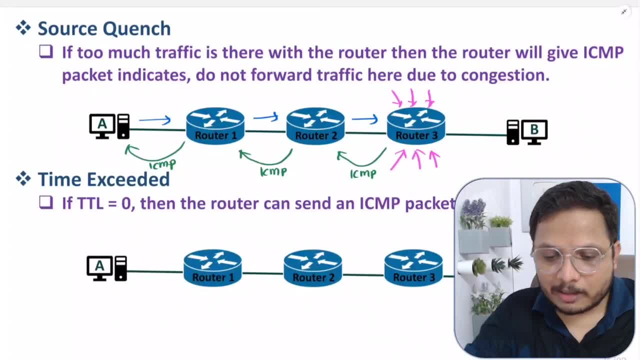 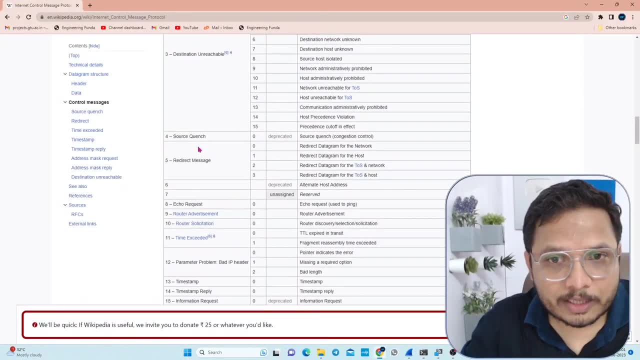 ICMP packet tells source quench. Let me show you that. let me show you that on my Wikipedia page, so that will give you more clarity. see source quench. see this source quench. so that explains congestion control. right? so I have told you like, if router is having too much congestion, then 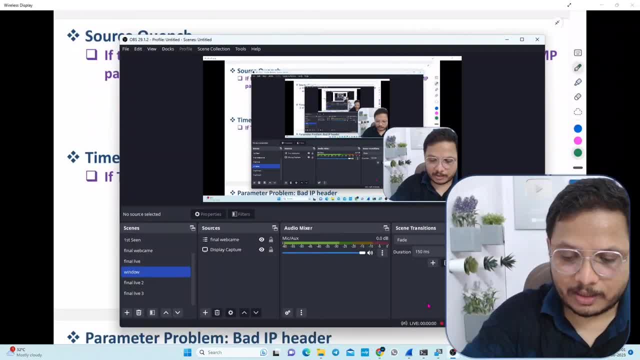 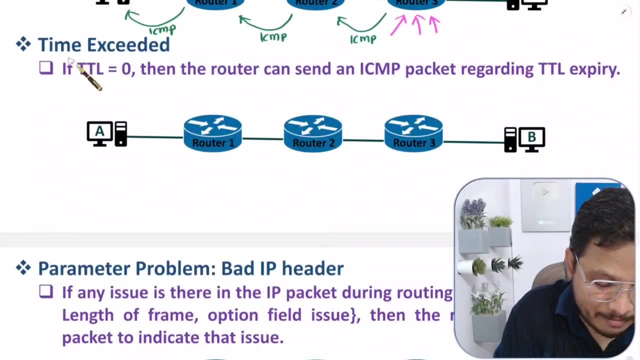 congestion control. that will be done by source quench Now. now let us try to understand one more essential usage, that is time exceded. so time exceded means what? Time exceded means what Time exceded means: now, frame cannot be forwarded further. time exceded means frame cannot be. 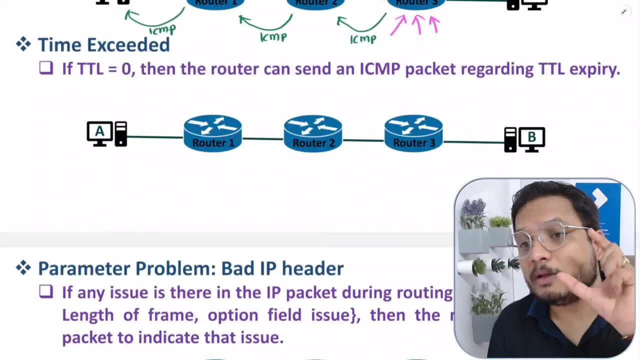 forwarded further and that we have already studied in IPv4, IPv4 packet format, in that I have told you like TTL, time to live, TTL if it is 0, if it is 0, then further hoping is not allowed. Let me show you one practical example. like right now I am having one frame right and 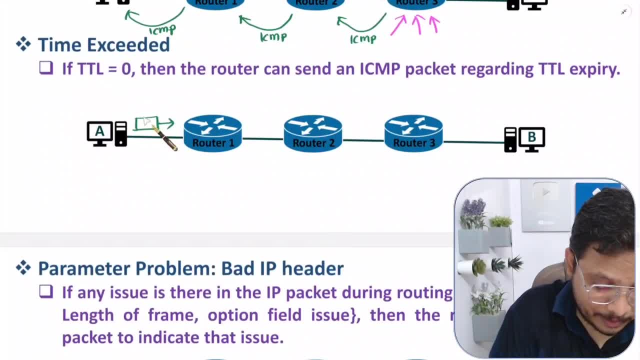 that is what I am forwarding over here Now. what will happen is like, for example: right now, if TTL, TTL is equals to 1 over here, right, when this frame comes over here, at that time this TTL will decrement by 1, right- TTL will. 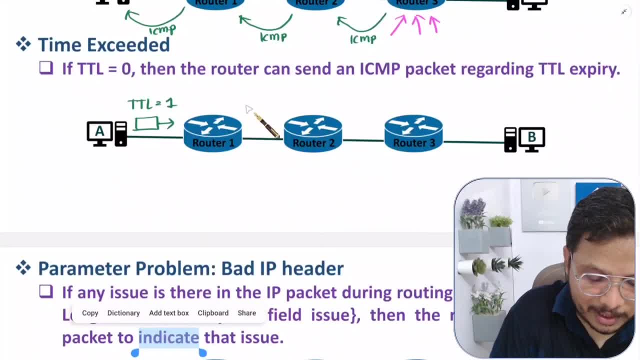 decrement by 1, so it will become 0 over here when it reaches over here, when it reaches over here, it will become 0, and as if TTL is 0, then further transmission is not possible. so this router 1, this router 1 will do what it will give, it will give ICMP packet over. 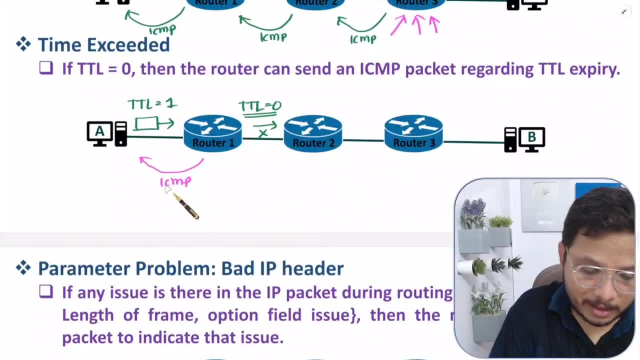 here and that ICMP packet explains what time exceded because of TTL is equals to 0, so this host will have to forward this frame again, right? so TTL field that explains now further transmission is not possible, but ICMP tells you can retransmit it. the reason: 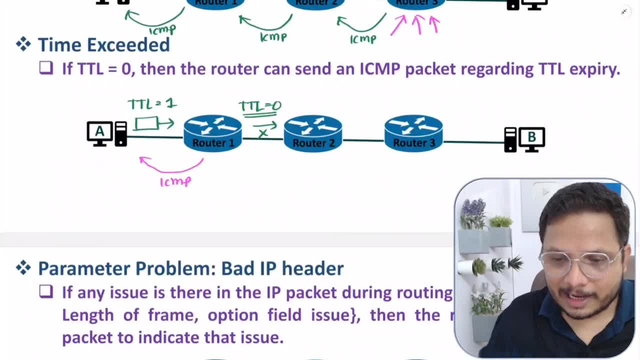 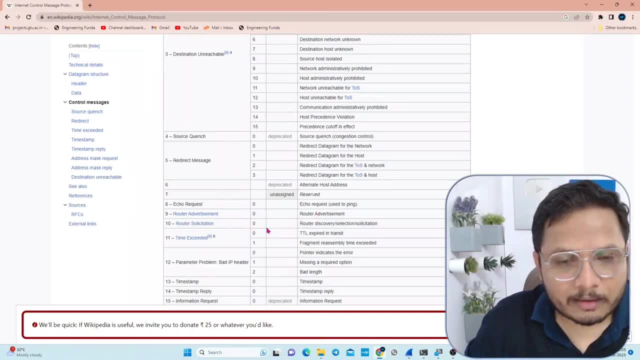 is now. it cannot be forwarded further. See. So these are the right. let me show you that on my computer screen with Wikipedia page, so that will give you more clarity. See here. time exceded. see this one. so it is having. it is having type. it is having. 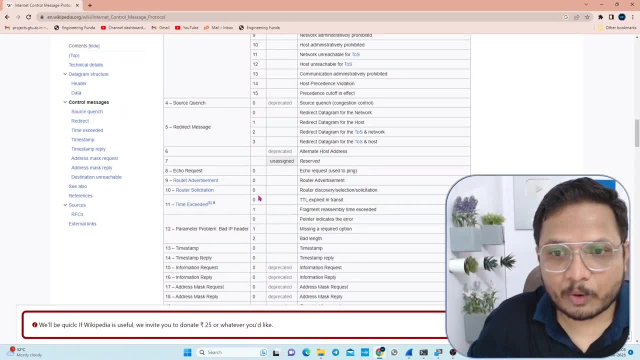 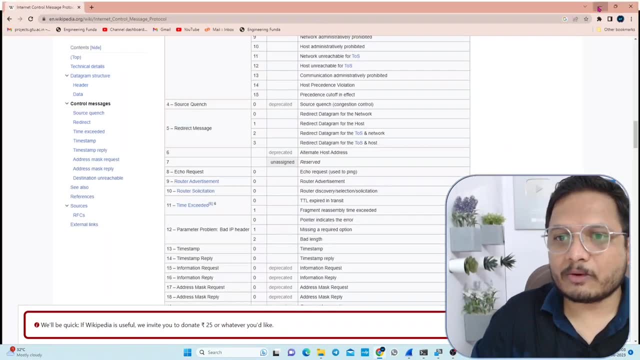 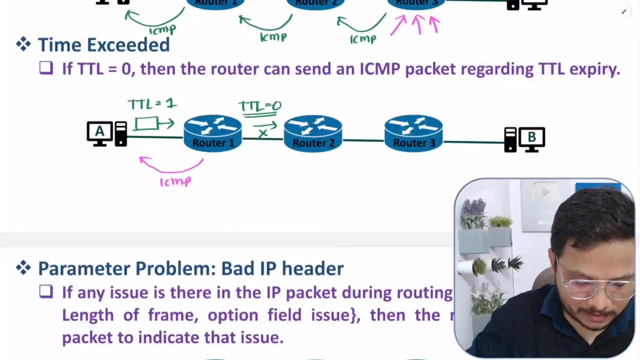 type 11 and there can be two types of code, right, so TTL expired. that that could be the reason over here. so this is how. this is how this reason is there. Now let us have next point Of this, which is parameter problem. so let us try to understand first what is parameter. 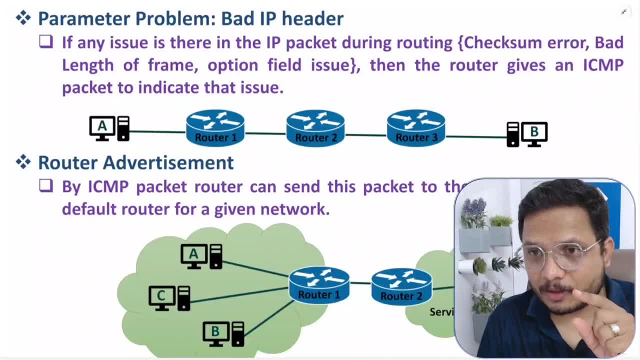 problem. see, there can be bad IP header. let me explain you how see, for example, as if I say: you are forwarding one frame from A to B. so whenever frame is getting transmitted via medium, there is always possibility. there is always possibility that there can be some. 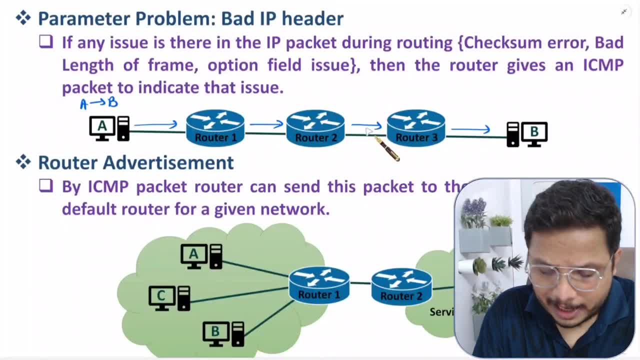 issues in data of frame And in majority of cases you will be observing those issues will happen in IP header. the reason is IP header will be identifying checksum right. so, for example, as if I say there is some issue, there is some issue right and because of that this router is observing. 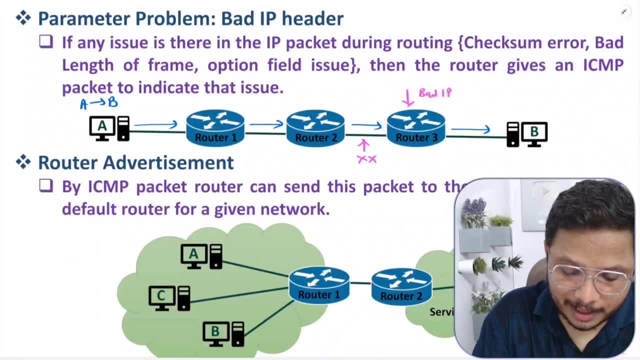 this router is observing bad IP header. So as if this router observes there is a bad IP header, bad IP header means there can be issues. There can be issue of checksum error, there can be issue of bad length of frame, there can be issue of option field issue, right, so based on that it will identify. okay, there. 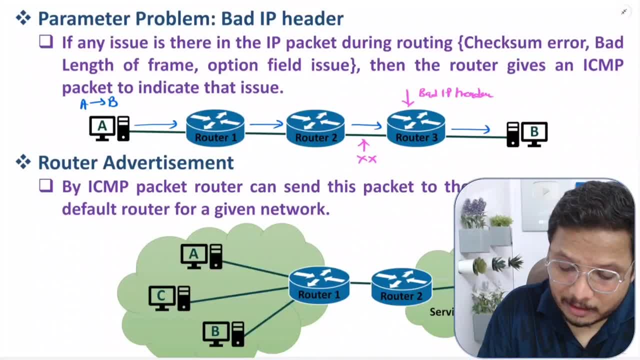 is issue of bad IP header and based on that, what it does is it gives ICMP reply, it gives ICMP reply to transmitter, it gives ICMP reply to transmitter and this reply says what this reply says. you will have to send this frame again, So let me show you that on Wikipedia so that will give you more clarity. see here with: 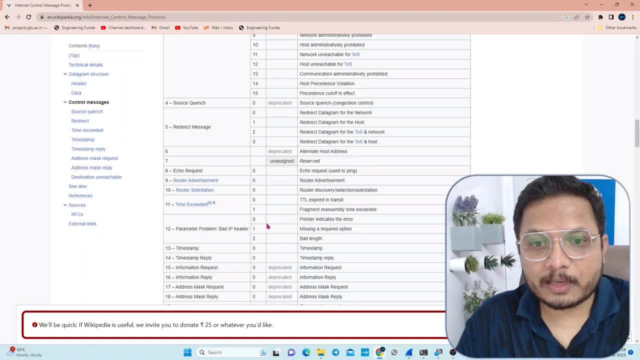 parameter problem. you see there can be three reasons. So here type and code that is there with us, right. so there can be bad length, there can be error as per checksum, there can be missing required option. So based on that we can identify there can be issue and those issues will be indicated. 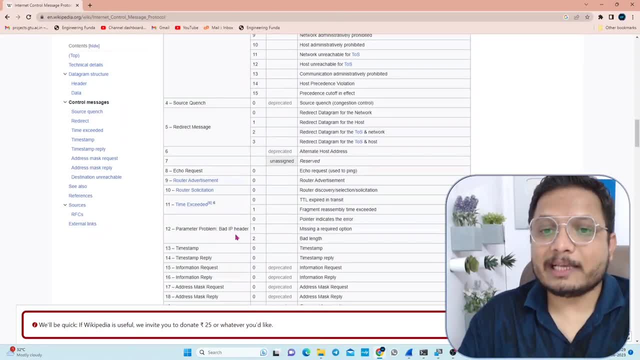 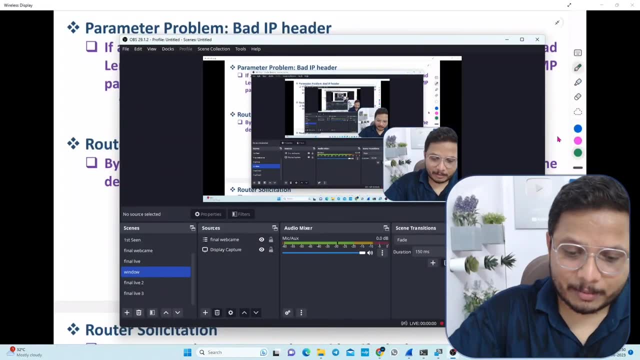 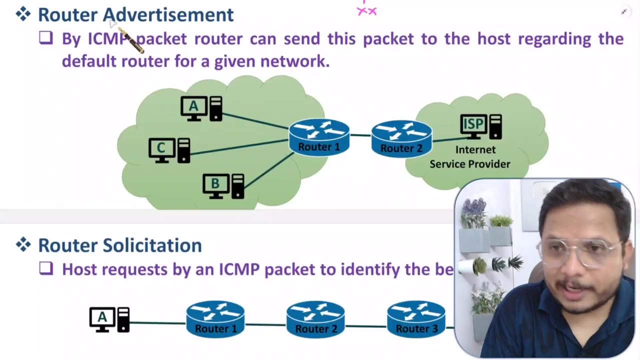 by those issues will be indicated by that ICMP code and type field. right Now let me show you another parameter, so that gives you more clarity. see router advertisement. So router advertisement that I have already explained right, for example, in this network: 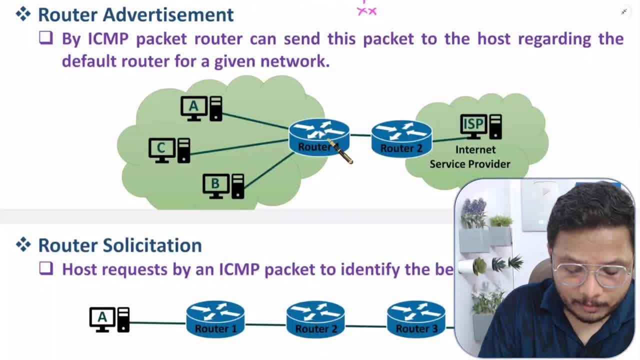 for example, in this network, let us say router is knowing this host are having best possible route via router one, Then router one will do what Router one will do: advertisement. like router one can forward frame to host A, that is ICMP frame, which indicates this is the best router which is there for you. 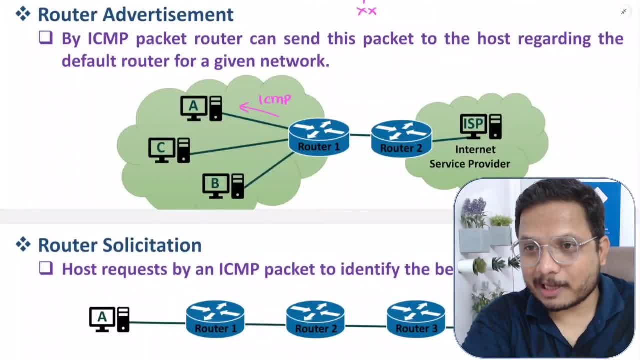 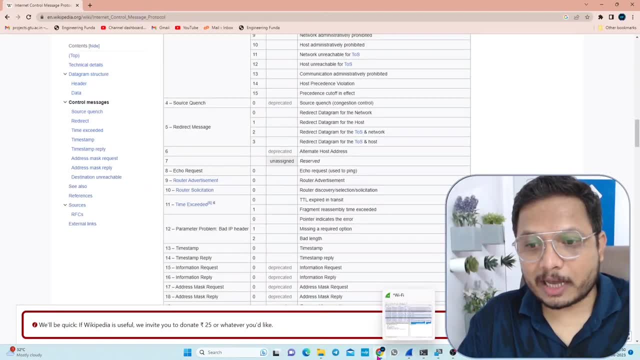 Like you see in my computer. I have received it, So luckily I have received it, so I think I should show it to you. see, here in Wireshark, I think I should show it to you see: router advertisement right. 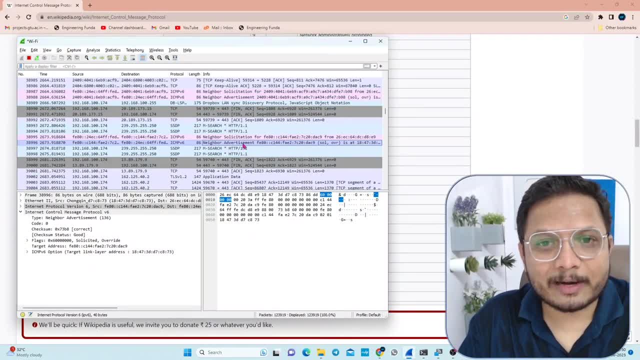 So router advertisement means what this router is doing advertisement It says: right now I am the best possible router for you, so you should be handling your traffic via me right. So that that has been indicated by this ICMP frame right. 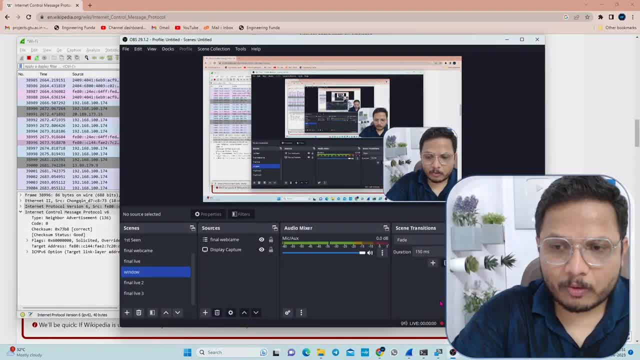 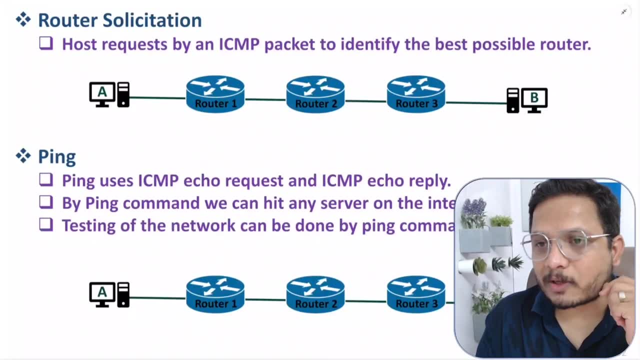 So I think now you are having more clarity regarding how. how we can have router advertisement right Now. similarly, we have router solicitation, So router solicitation, So router solicitation, So router solicitation. that is what that explains here. host is identifying best possible. 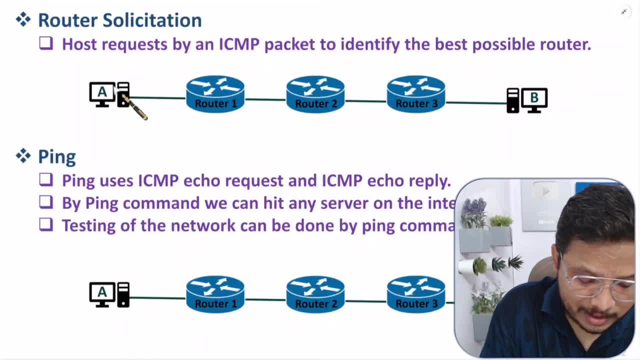 router. Let's see, for example here: host host A wants to find best possible router, then host A will send ICMP frame. host A will send ICMP frame and it indicates to router one: are you the best possible path for me or not right? and based on that it will receive. 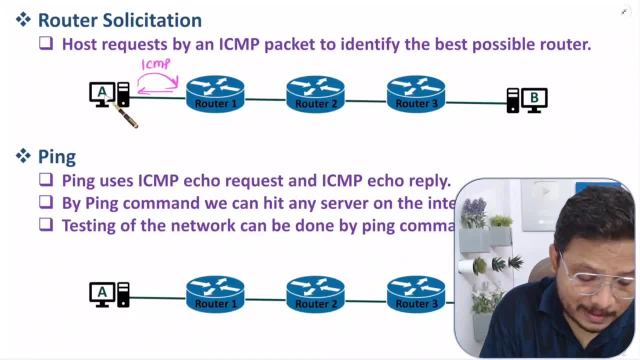 it will receive acknowledgement. So here A is asking for best possible path to router. that is what router solicitation, right, that is what router solicitation ICMP frame. Now let me explain you few very essential parameters, like what is ping and what is trace. 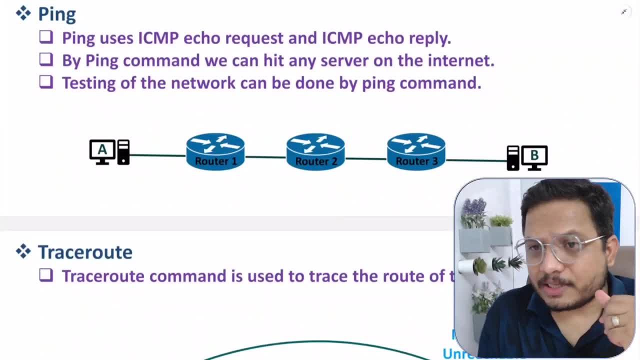 route. The reason is as, being a network engineer, you should be having idea about what is ping and what is trace route. and why should we have it right? See ping that uses ICMP echo and ICMP echo reply. So ICMP echo request and ICMP echo reply. that can be done by ping. I'll show you practically. 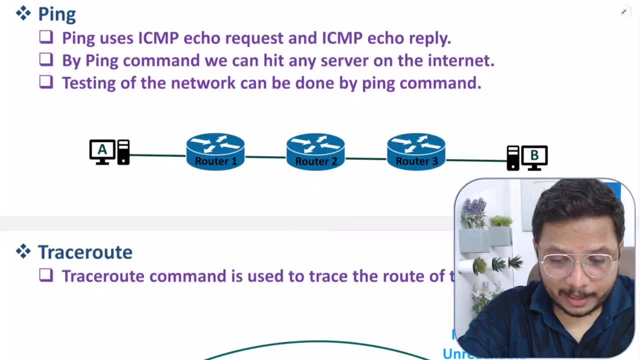 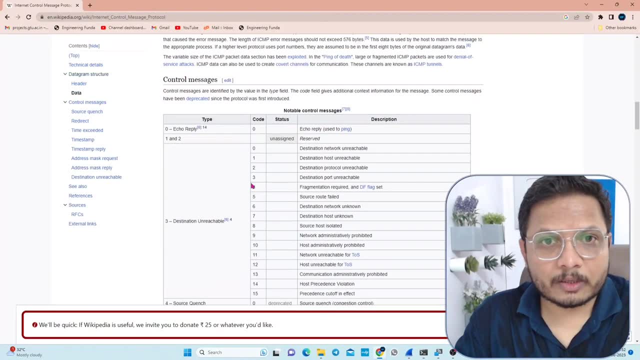 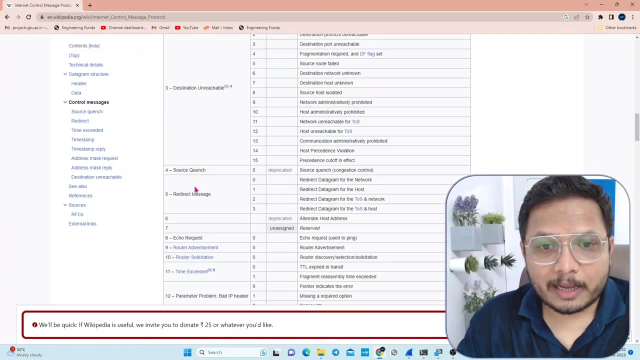 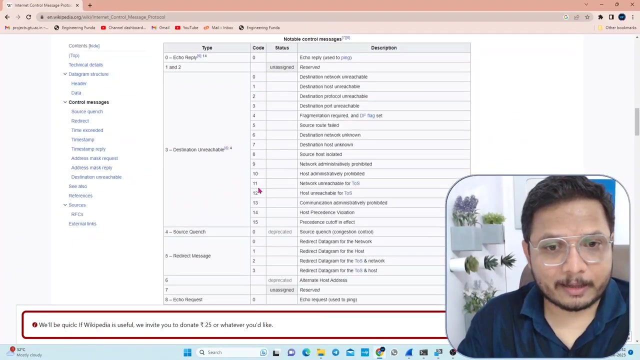 right. First of all let me show it to you on Wikipedia and after that I'll show you practically on my computer. So here you see. ICMP echo reply. So that is having code zero, type zero, And ICMP echo request. that is having eight and zero type and code, right. 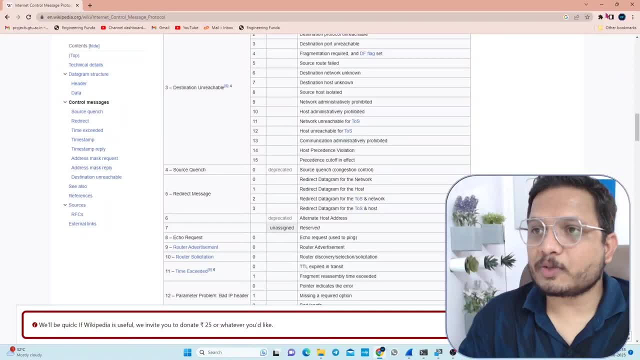 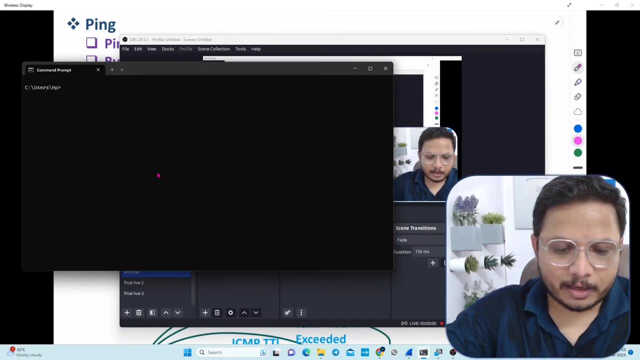 So this is what we can have it by having ping. So let me show you how we can have it. So for that you'll have to open command window, and this is Windows computer. So in Windows computer, in Windows computer, you'll have to write ping, and then you can. 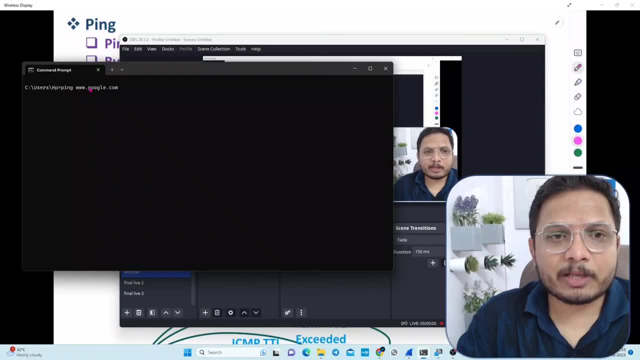 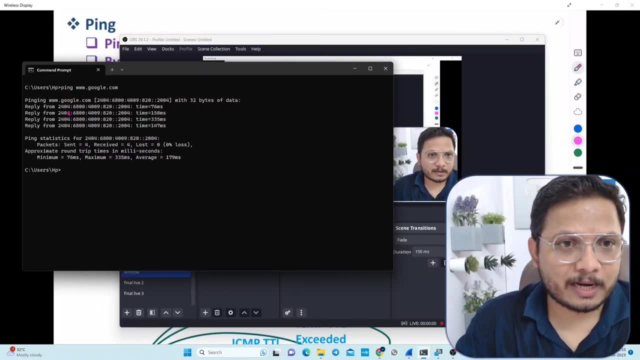 write any website, So as if I write wwwgooglecom, Right. So if I write wwwgooglecom after ping, then what will happen? you see, it will be forwarding frames, right, And these are IPv6 frames that you can observe. 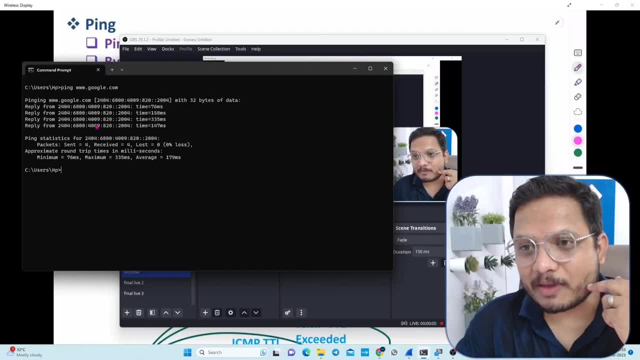 And I have told you like. see, we were been communicating with IPv4, but nowadays IPv6, that is getting popular, And these are IPv6 frames right Now. see what it indicates. It indicates how much time that it took to reach out to Google. 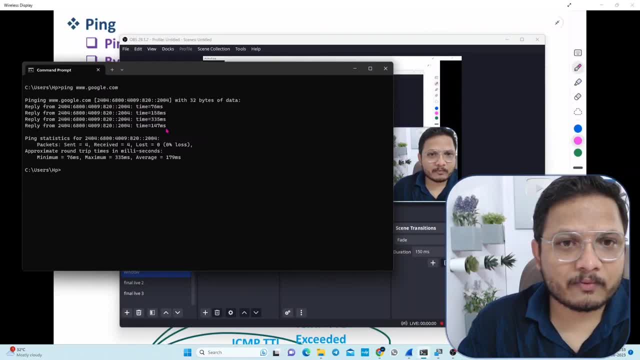 So first frame, second, third frame, fourth frame, fifth frame, fifth frame, sixth frame. fifth frame, sixth frame, Right, Third, fourth. See, this is how reply comes right. So, with respect to time, how much? how much time that that my computer to to get onto? 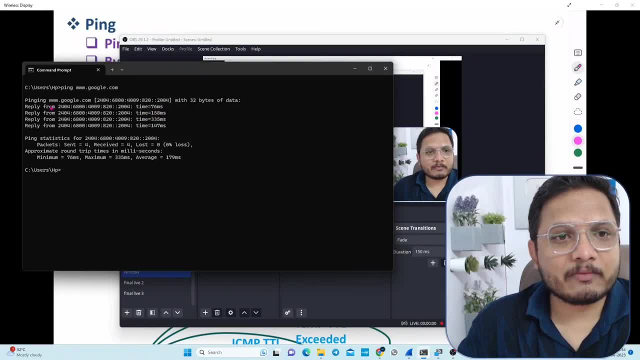 Google server: right. So 76 milliseconds with first ping, with second. it took this time right. So here I can understand, like how much time it takes to have that route to that given destination. that I can understand based on ping command. 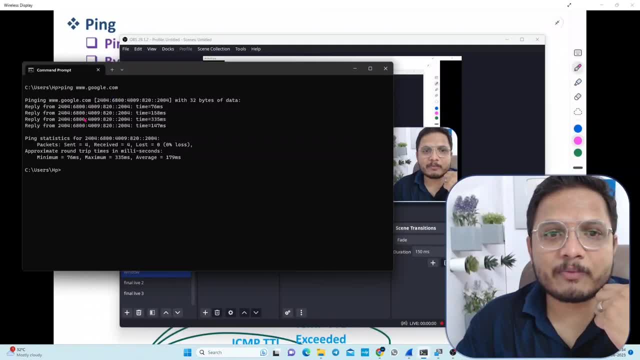 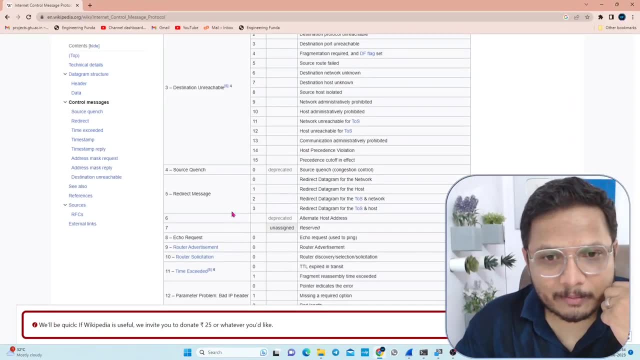 Right Now, when you perform this ping command At a time, it will be forwarding request and it will be receiving reply. right And that request and reply. that request and reply: see request. that will be this and reply that will be this. 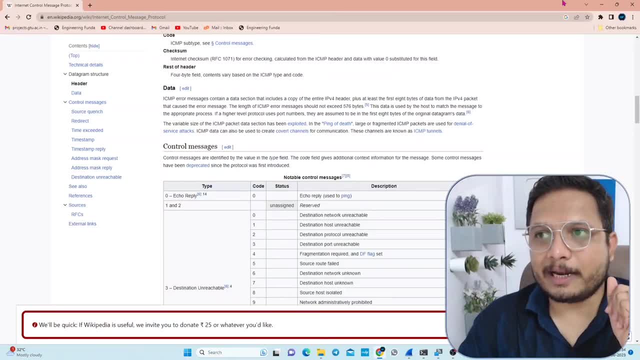 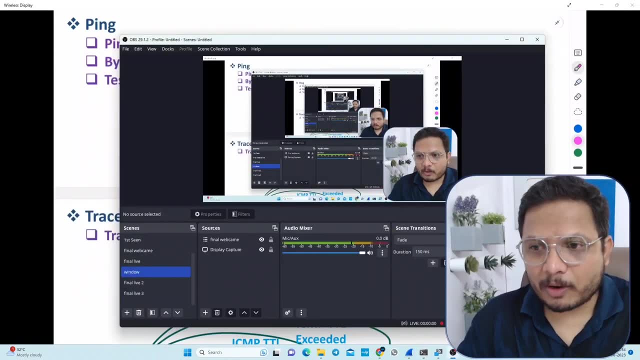 See, as per this type and this code, it will happen right. So in ICMP packet format that we can understand. So probably I think now you are having fair enough idea about what is ping. right Now let me. let me show you how trace route is there. 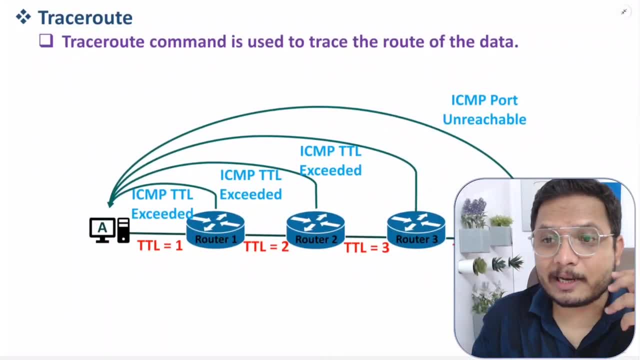 See, This is an amazing thing by which you can understand exactly what is happening in your computer as per computer network, Like see, for example: if I say what, what could be the path by which I can reach, is to Google, then that I can find it by having trace route. 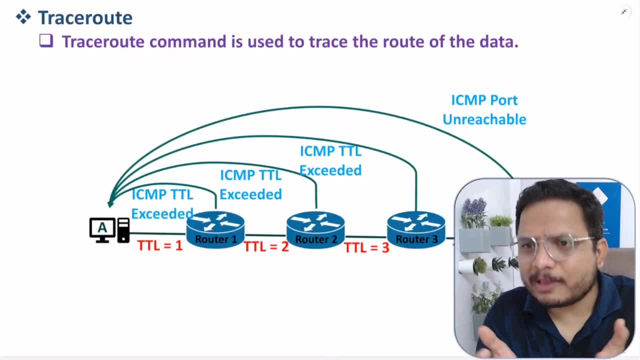 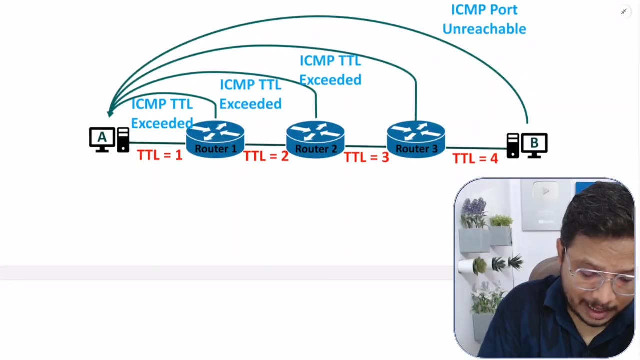 Like when I, as and when there is some issue in any small network, even by having a trace route, we can identify what is. what is the exact path at which there is some issue. Right, Let me show you how. see, for example, here, here, as if, as if I want to identify what. 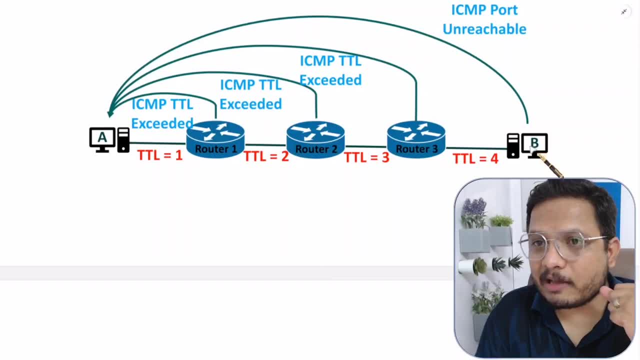 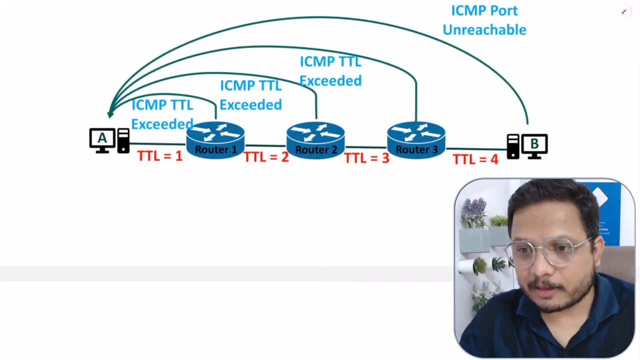 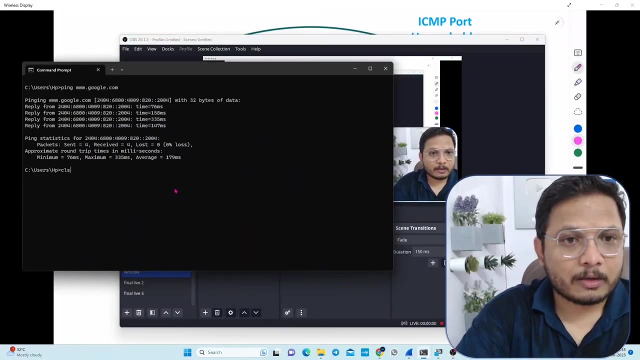 is my path from A to B, then I can identify by having trace route. Let me show you practically first. after that I'll explain you how it is happening, Right? So here on command, you see, I'm I'm writing trace RT. 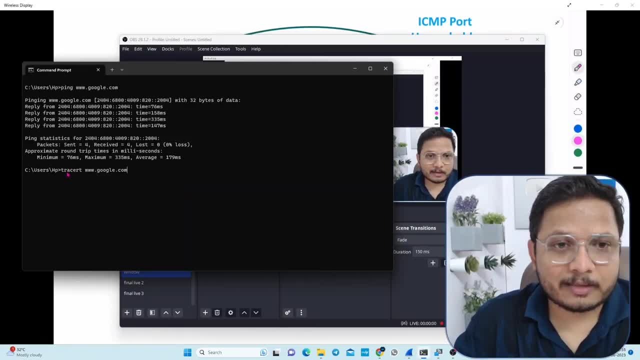 Right Right Right Right. See, this is Windows computer, So in that you'll have to write trace RT. If you are having Mac, then you'll have to write trace route. So trace RT, then wwwgooglecom. So I just want to find a path. 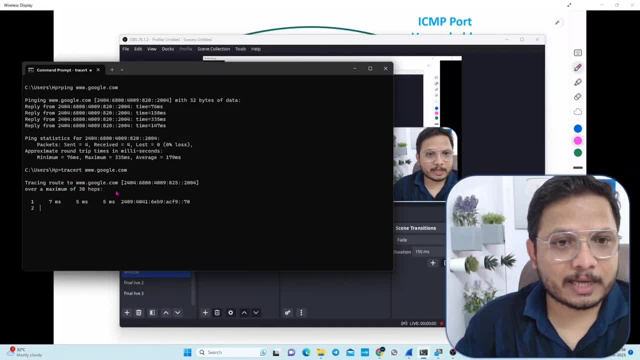 Now let me, let me see how trace route is there. You see what. what is written first Over over a maximum of 30 hopes means in between 30 hopes are there. In between 30 hopes are there Right Now. you see, some requests are getting timed out and some requests that is happening successfully. 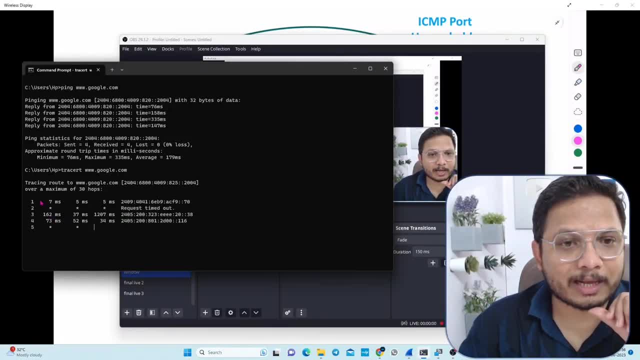 over here And it is showing me like what? what are the path which is happening right now in between me to Google server, right As Google server is very far from me. obviously there can be timeout. The reason is ICMP protocol is not compulsory. 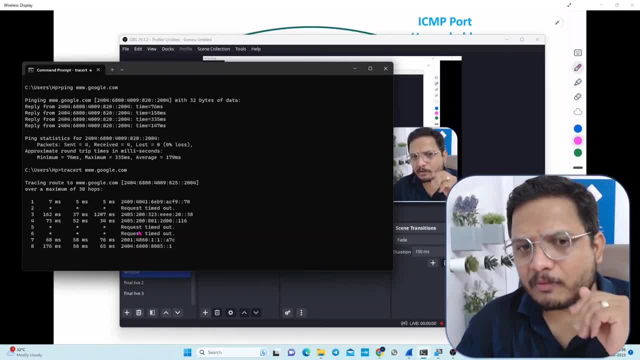 I have told you, but for small network we can communicate. My network is very small. I'm having just five computers, Five computers only, right. So I don't think like trace route will function over here with my network. But if you have network with hundred computers then definitely this will be helpful, right? 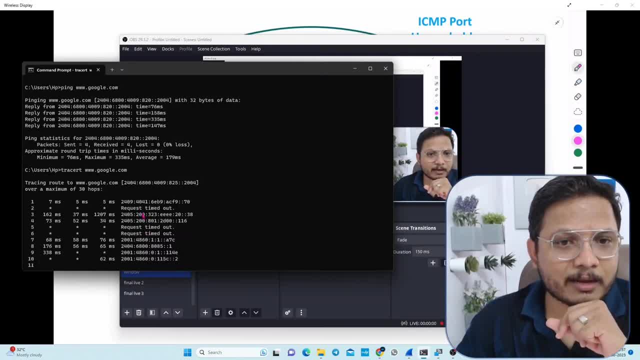 To trace a route. You can observe here some routes that has been indicated over here. some some routes are having the request timeout So I can identify like what are, what are the IPs right Which is available over here during my route. 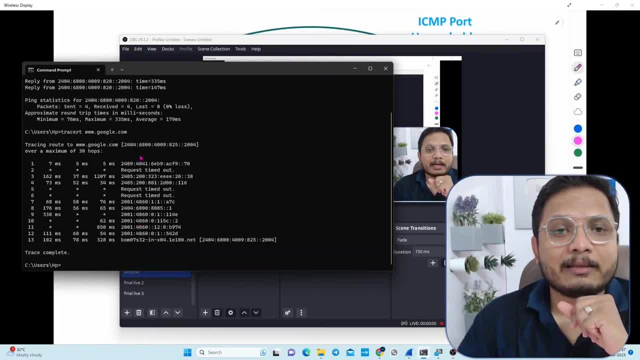 And Based on that, I can. I can. I can understand, like, how exactly frame is getting transmitted, now, how it is happening. Let me explain you that. that gives you more clarity right Now. you understood what, based on trace route, you can understand, like, what are the possible? 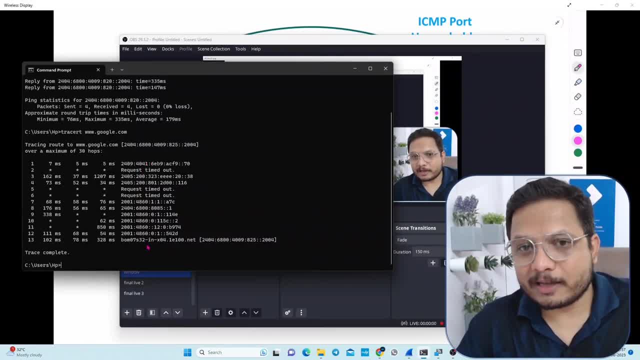 paths by which my frame is getting routed right, And that is that has been given over here in sequence. See, this is. this is not the exact thing right now, but if it is about five to six route or Six hopes, then definitely you can say it will be correct one. 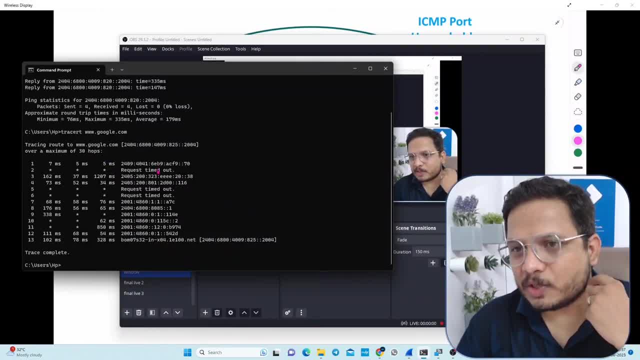 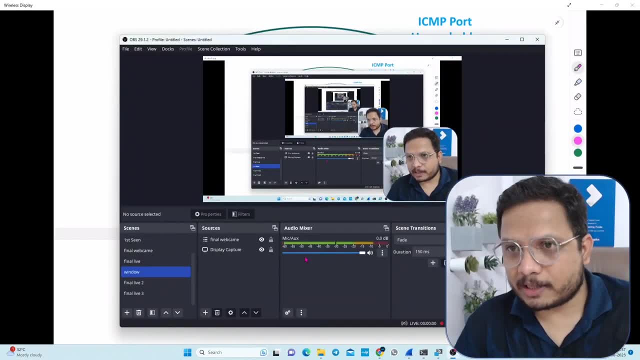 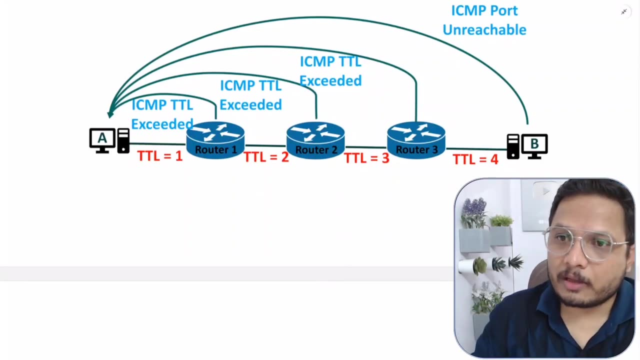 If it is having more than 30 hopes, then there definitely there will be some issues, right? The reason is there can be multiple paths. as number of both hopes increases, then you will be having more choices of path, right? So let me explain you first how, how this command is working. 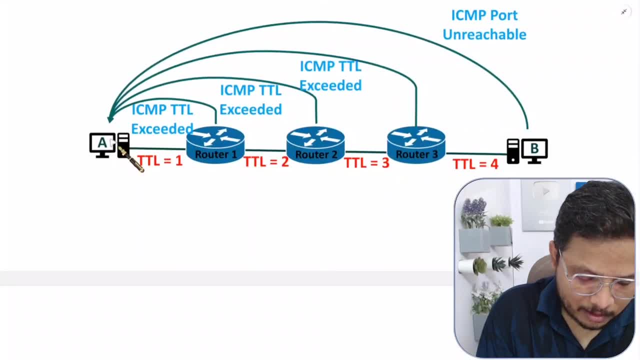 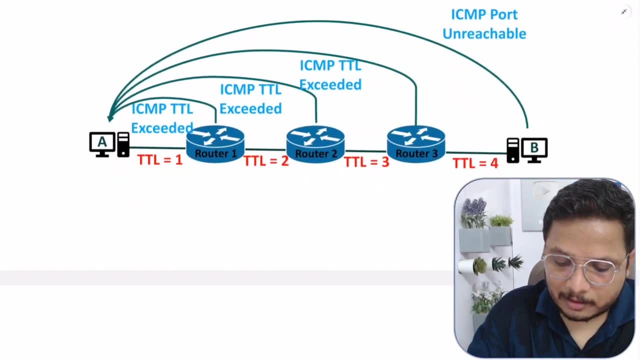 So for that, you see what is happening here is here Post a. see, this is my computer, So this is, this is me, And let us say this: host V, that is Google, This is Google, right? So what host A is doing, host A is writing trace route, trace route or trace R T see. 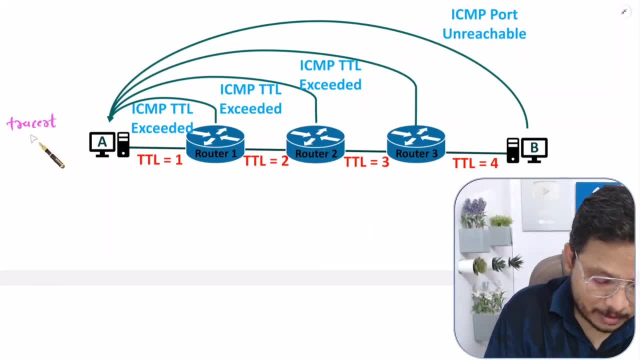 trace R T- that is there for window system and trace route that is there for Mac. So trace R T and then space, And then, as if I write googlecom right, Googlecom, Right, Googlecom, Then I just want to find a path to reaches to Google. 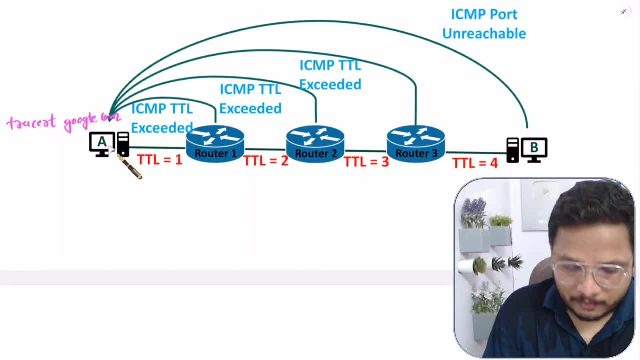 Now how it is happening. You see see first. first, this computer A will send one ICMP frame. This computer A will send one ICMP frame. With this frame it will set TTL time to leave field that is equals to one. 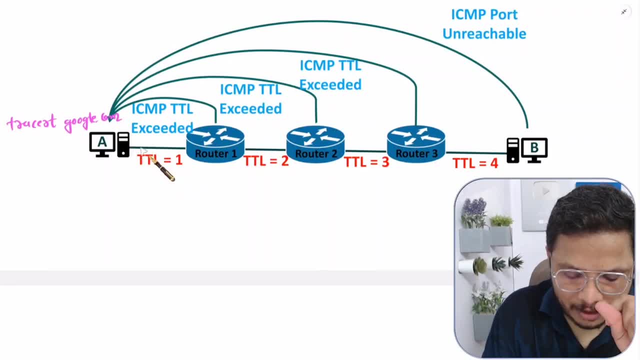 So what will happen when this, when this uh frame reaches over here, This TTL will become zero. And as TTL will become zero, this router one will forward what ICMP TTL exceeded frame. So router one. so so my computer will get to know: like okay, first router, first router. 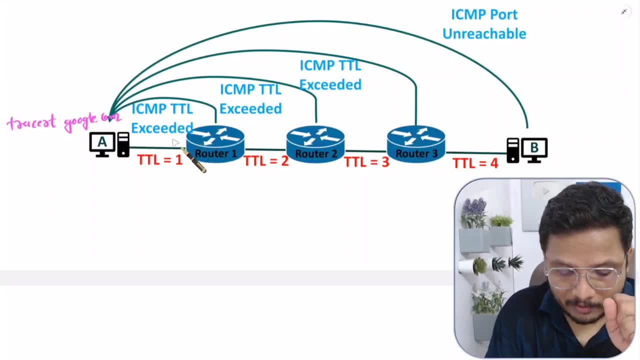 has forwarded ICMP TTL exceeded. So my first, first hope, that is this: Now, next time this computer will set TTL is equals to two and it will forward frame, So it will go to router one At that time, this TTL that will change this from two to one. 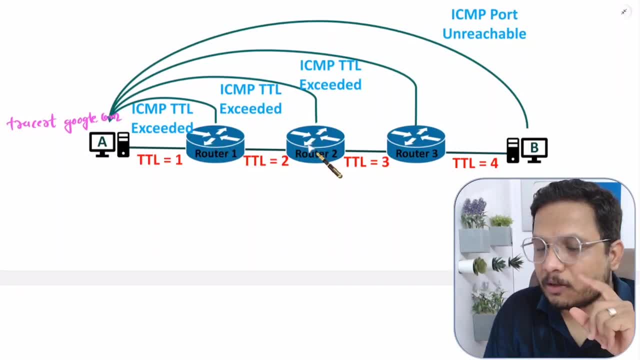 And then again it will reaches to two and TTL will change this from one to zero. So again here TTL will become zero. So this router two: it will forward ICMP. TTL exceeded reply to host A. right. Next time now host A will send what? 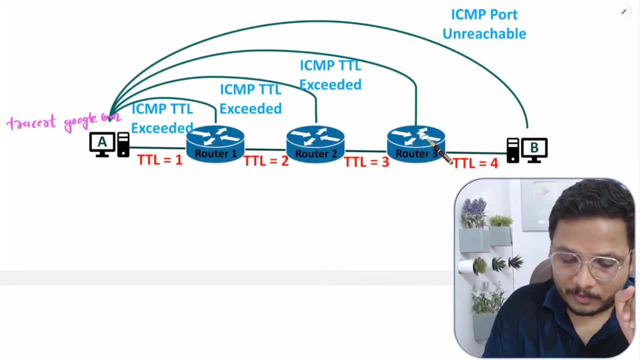 Frame with TTL is equals to three. So timeout will happen over here, right, But at last, when it comes to Google, at that time, at that time you cannot forward. TTL is equals to four. Why? The reason is: if you set TTL is equals to four, you are writing googlecom. 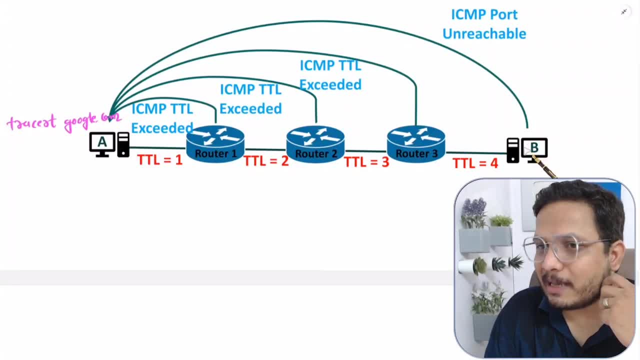 So request is already reached over here. So Google will not send ICMP reply over here. So for last hope, for last hope, what this computer will do is it will send a frame. It will send a frame, Okay. It will send a frame with destination Google, but with false port number. 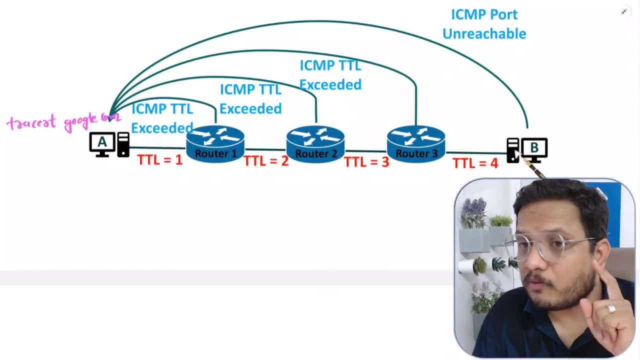 It will send a frame with destination Google with false port number And when it reaches to Google with false port number, Google will give reply: ICMP port unreachable. ICMP port unreachable to this. So this computer will get to know like: okay, Google is there after this number of hopes. 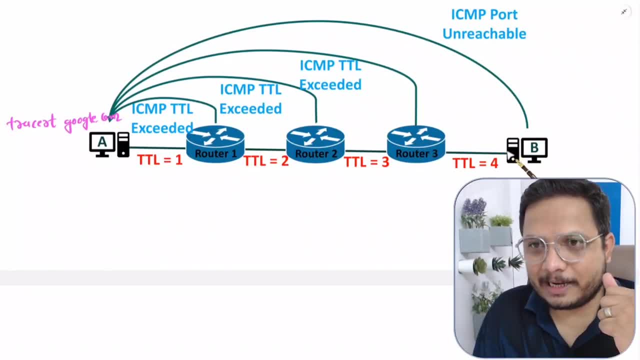 See, this is how things are happening practically right. So here few basic things that you should know. see here this computer is sending frames with. TTL is equals to one, two, three, And based on that it identifies how many hopes are happening over here. 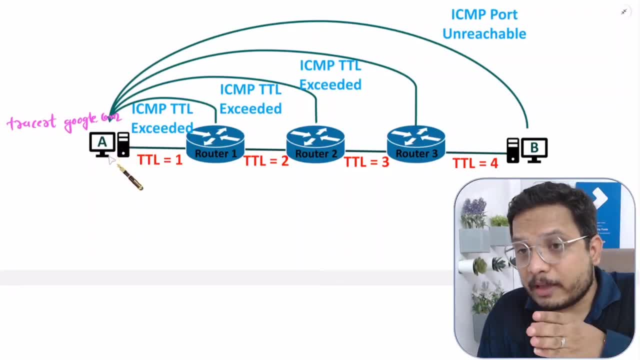 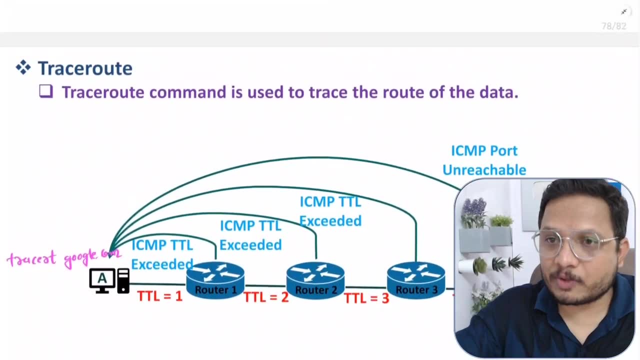 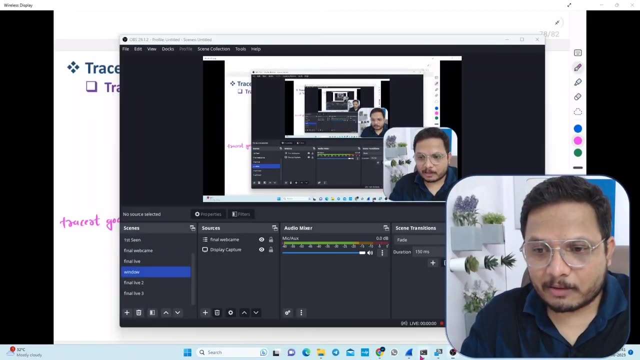 So, based on that, here this computer is observing what is the path by which communication is happening Practically. If you observe, practically, If you observe When it comes to, when it comes to a complex path, when it comes to complex path like 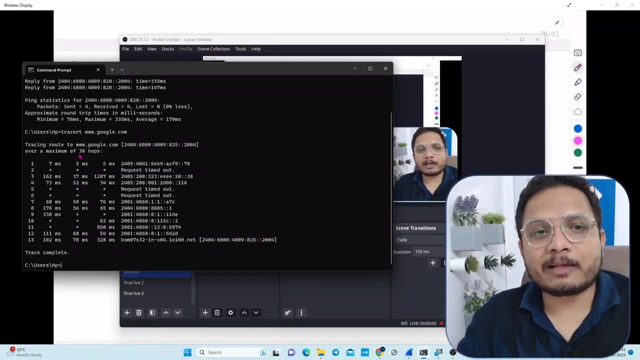 from India to USA. initially it have told like there can be. there can be over maximum of 30 hopes. Even it is not having an idea about how many hopes can be there. Why? The reason is: as you increase more number of hopes, obviously there can be so many paths. 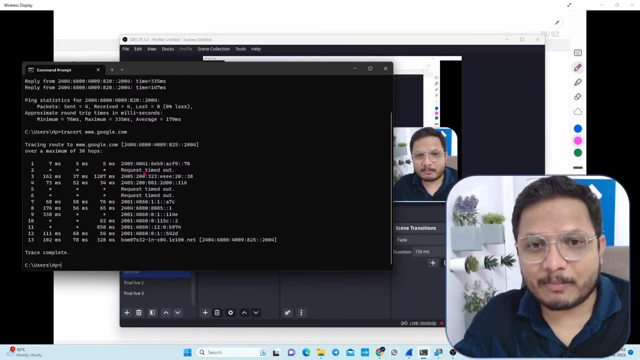 So when it was identifying path over here at the time, there was a request timeout. Right, There was a request timeout. Why that is happening? The reason is I have told you: ICMP. that is not mandatory. ICMP is not mandatory. 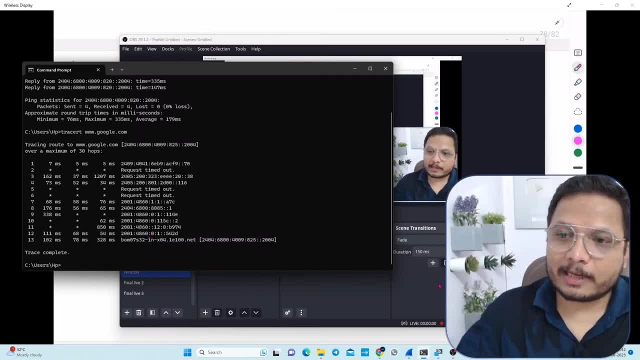 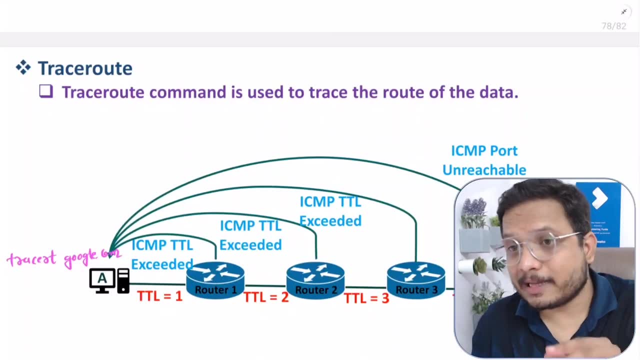 It is optional Internet protocol. internet protocol is unreliable service. Internet protocol is unreliable service And as internet protocol is unreliable service by ICMP, we can improve reliability Right. So it is not compulsory Every time. ICMP frames will come Right. 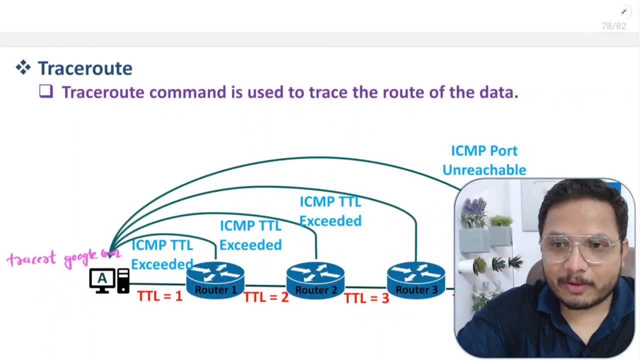 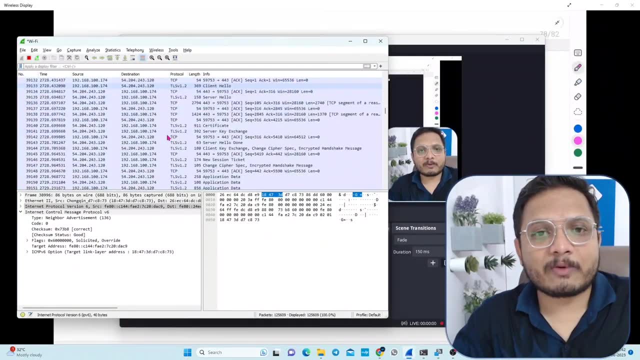 That is why. that is why what was happening, you know, like, when I was searching for ICMP frame, when I was searching for ICMP frame, it was very difficult for me. You can observe here: on Wireshark software, I do not find ICMP frame. 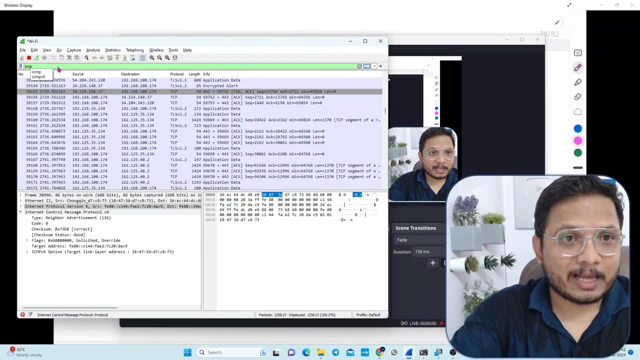 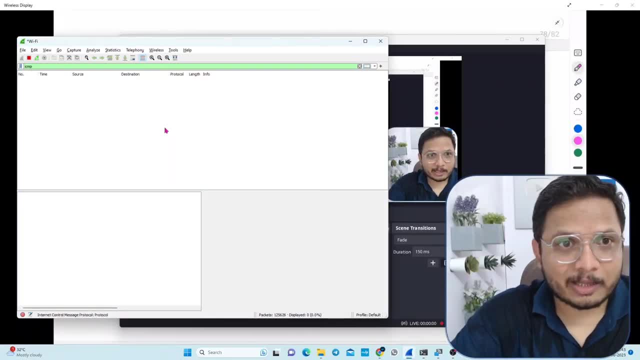 So here in filter I need to write ICMP And when I write ICMP you see ICMP that I am not receiving. But I have received few ICMP, ICMP along with version 6.. Right, I have received few with ICMP with version 6.. 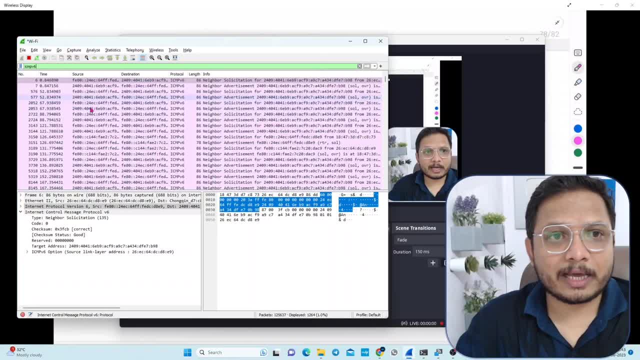 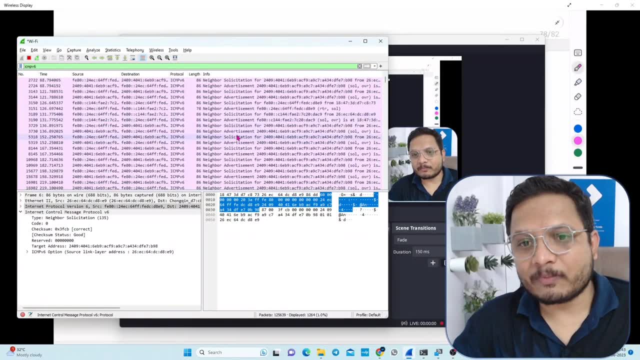 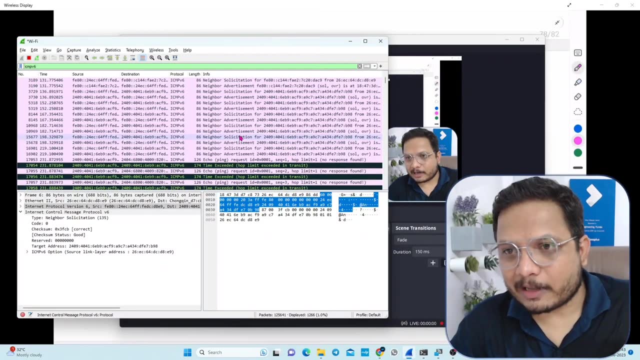 I have shown it to you Right Now. I just need to again. you see, ICMP with version 6, I have received so many And those were the regarding solicitation and advertisement. Now, solicitation and advertisement: that see, that is regarding advertisement of router. 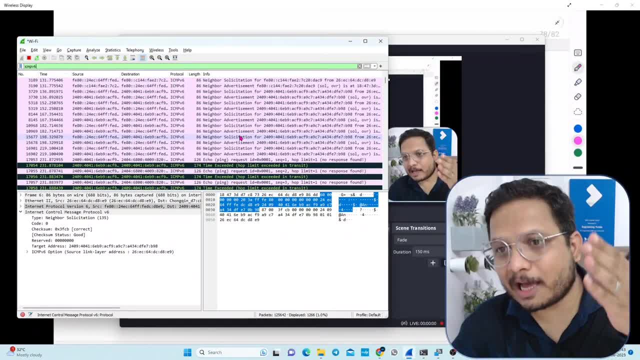 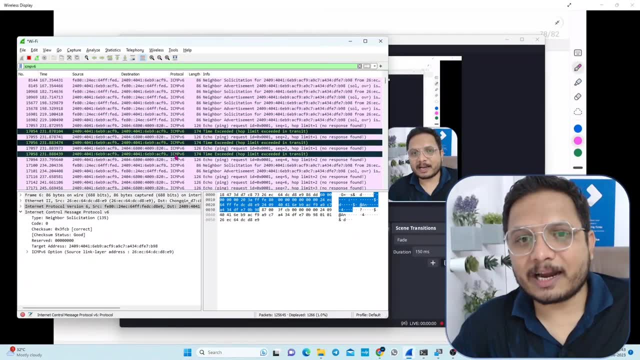 Right, And one frame that I am asking to my router like: are you the best router or not? See these two frames that I am receiving. Otherwise, if you observe, here I am not receiving any frames regarding ICMP, ICMP version 6.. 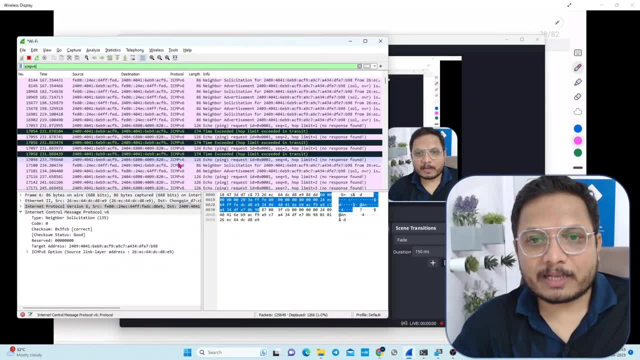 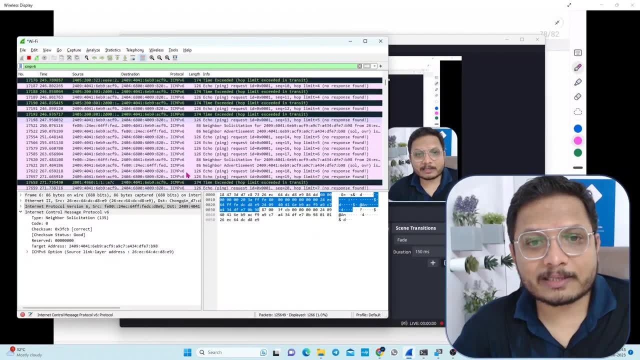 That is what I am receiving Right: ICMP version 6.. That is what I am receiving Right Now with majority of cases Right, And that is what I am receiving because of ping command that I have used Otherwise technically in my communication. there is no issue. 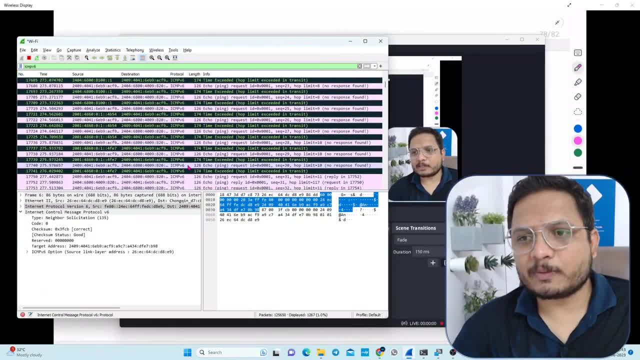 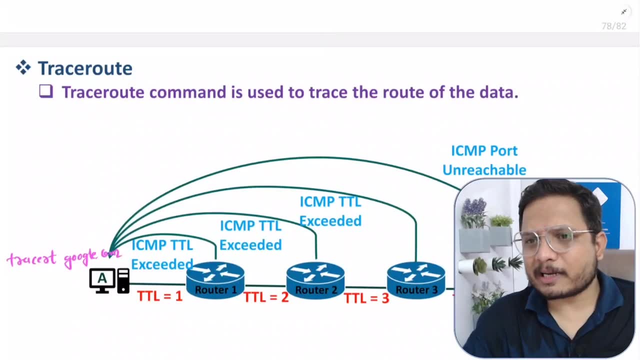 Why? The reason is: nowadays if you observe internet speed, then that is very fast, Right And very few chances of errors are there. very few chances of frame drop will happen And because of all those things, Probably In future you will be observing. 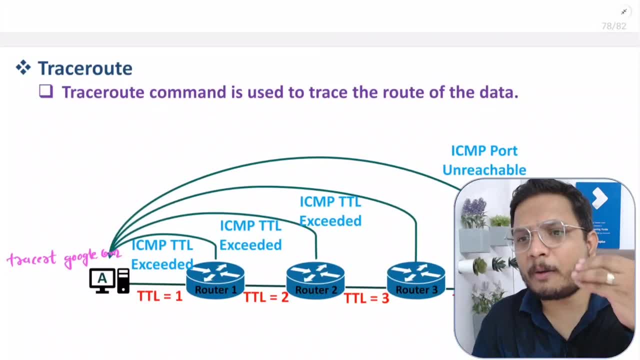 Internet will be very fast without error. we will be communicating. optical links are available in which there are very few chances- very rare chances will be there of error, But still error is possible. But as bandwidth is expanding, less errors are happening. 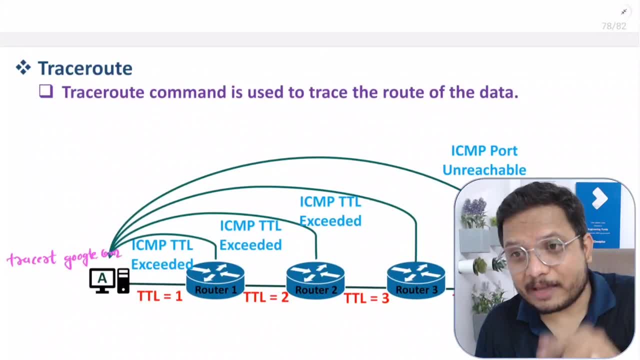 And that's why, even if you search for ICMP frames, very rare chances are there that you will be receiving it, And I was been searching for ICMP frame For two hours, Right, And I was not getting it, And I have received a few only, which were there regarding advertisement and solicitation. 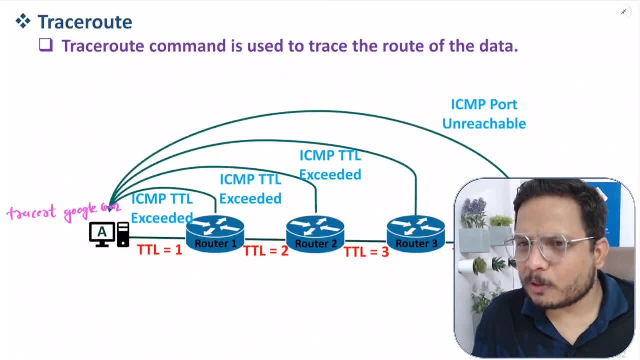 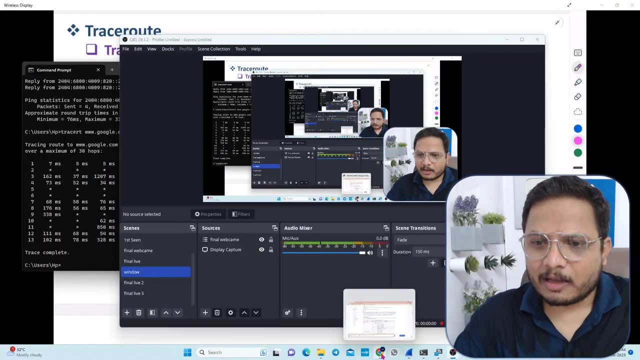 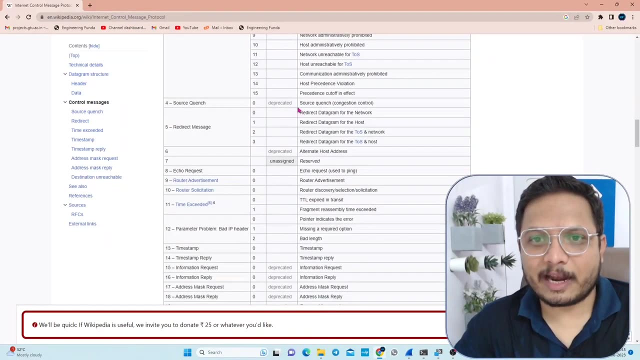 But still, to improve reliability of internet protocol, ICMP is essential. But still, if you observe few things over here, if you observe few things over here on Wikipedia itself- see what they are saying: Majority of things are depreciated, Right. 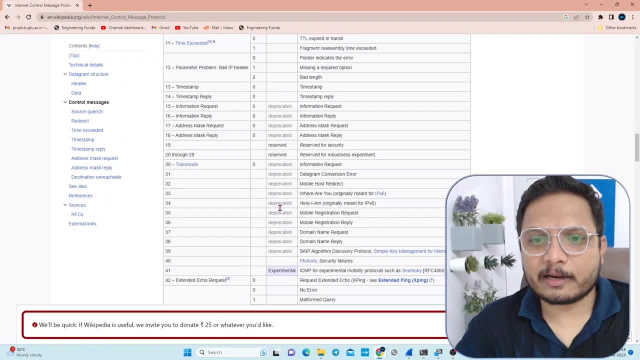 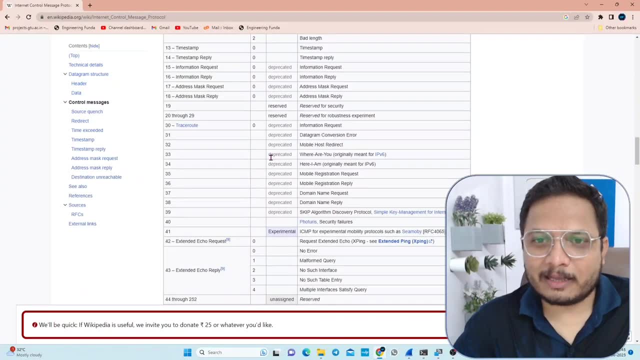 Majority. You see, depreciated, depreciated, depreciated, Right. If when I was studying, like you, in engineering, at that time, when I have seen that on, when I have seen that on Wikipedia, at that time very few were depreciated. 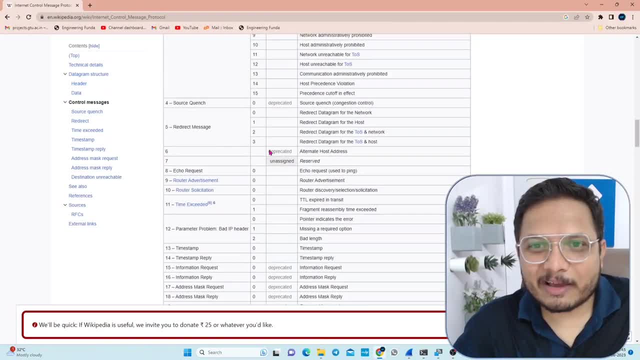 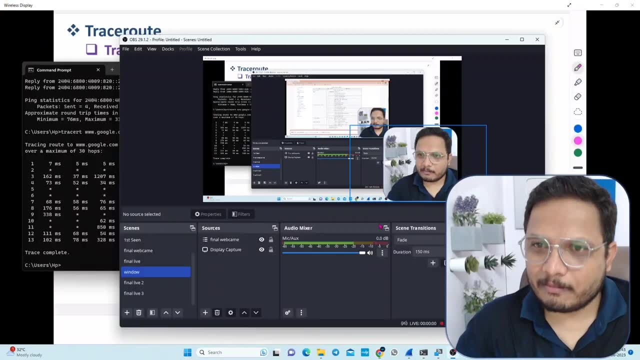 But nowadays this depreciated. that is increasing on Wikipedia, even Right. What it means. in future you will be observing majority of ICMP that will be depreciated. Right Majority will be depreciated. The reason is: nowadays internet becomes reliable, relatively reliable.